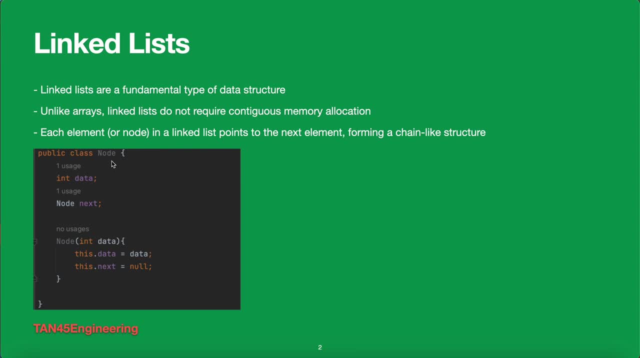 pointer in the same node, Like, for example, in this node. we have created a simple node. we have data, that is the value of that element, and then it stores the address of another node. Okay, so we'll understand that quickly. Okay, And similarly, the next node will hold the address for the next node and then the next one will have the address for the next one. Likewise, a quick comparison with the arrays. Arrays store elements in contagious memory. 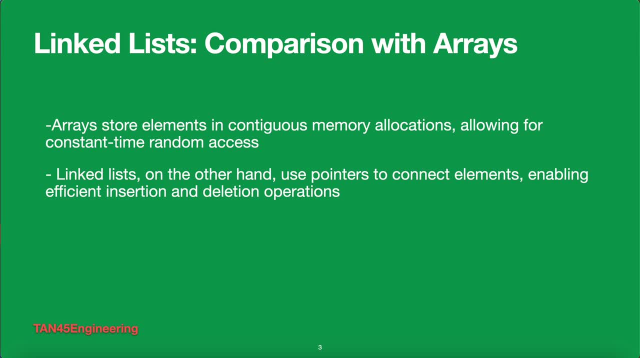 Allowing for constant time random access because, since they are in the contagious memory allocation, we can do the indexing on them and we can directly fetch random elements at constant time. right, If you want to fetch the fourth element, we can directly do nums of three. three is pointing to the fourth element, because indexing again starts from zero, zero, one, two, three. it pints to the fourth element. Bueno, there. 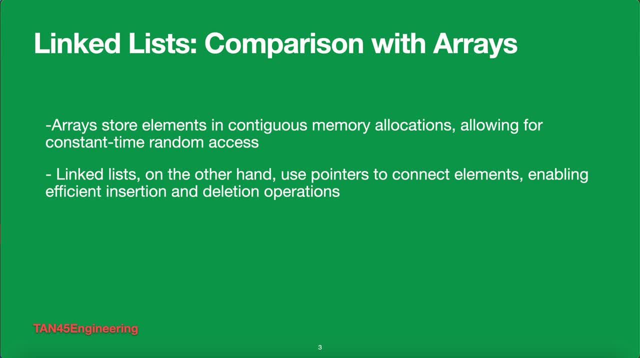 Linked list, on the other hand, uses pointers to connect to elements enabling of number, em, Це, Because indexing for material elements starts from efficient insertion and deletions. so let's look at this point. we'll come. come to this point as well. okay, so we saw that linked list are fundamental type of data structures, unlike 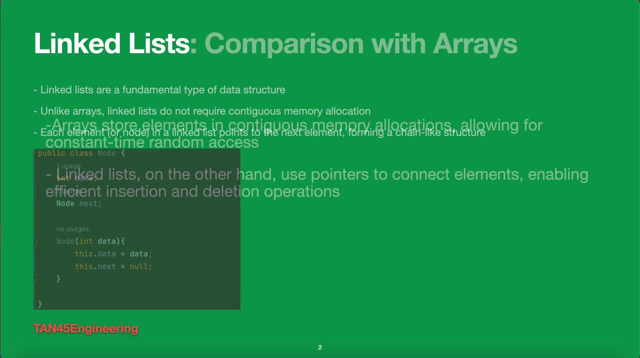 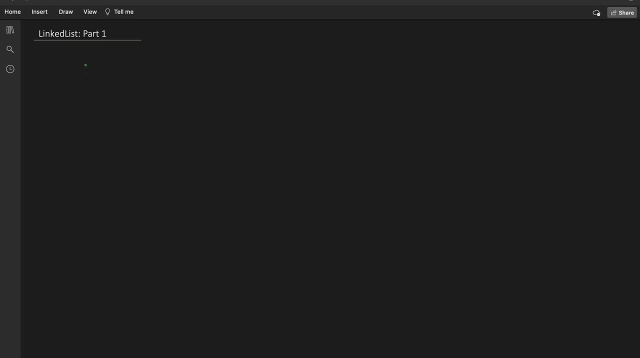 array. they do not require contagious memory allocation, okay. okay, let's understand linked list here. so, just as a quick review, let's say we have, oh, not this. yeah, let's say we have these numbers: 1, 3, 5, 7, okay, and first let's say we store them in in an array. okay, so how array? 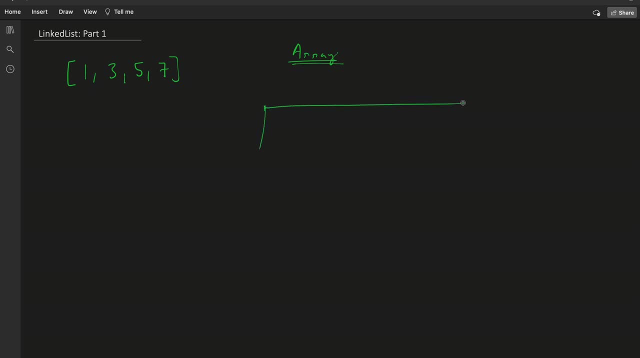 will store them is: let's see that this is memory in the system. so our 0th index is here. let's call it 1000. okay, so this is our 0th index: 0. so this is 0th index, this first index. second, 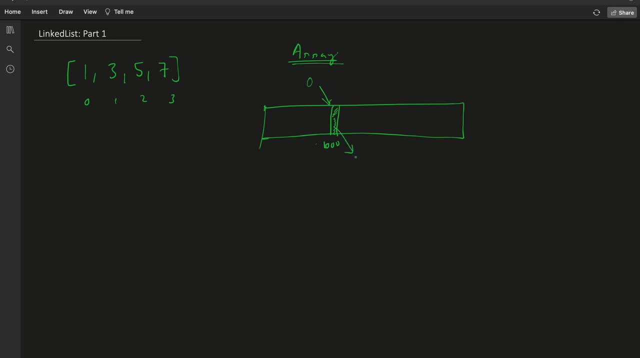 index. third index: it will have the value 1, then right next to it will have the value 3, then 5 and 7. okay, wait, this is index 1, this is index 2 and this is index 3. okay now, if I want to fetch the. 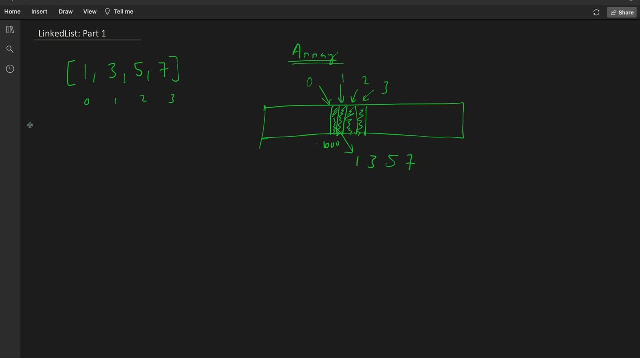 first element. let's say, the array was given the name as nums. so if I want the first element, I can simply say nums of 0. if I want the third element, I can say nums of 2. right, that will fetch me 5 nums of 2 on the second time. this is how these numbers would be stored in in an array. 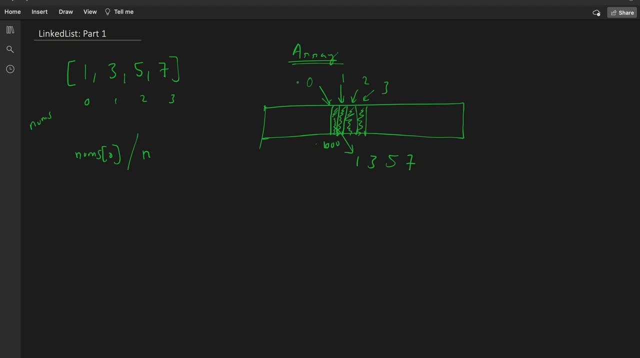 right now let's go back a little. okay, let's see how will we store them for linked list. okay, so linked list, as the name suggests, they are linked. first let's look at their memory allocation. okay, if 1 is stored here, so we'll have two sections to it. okay, first section would be the data. 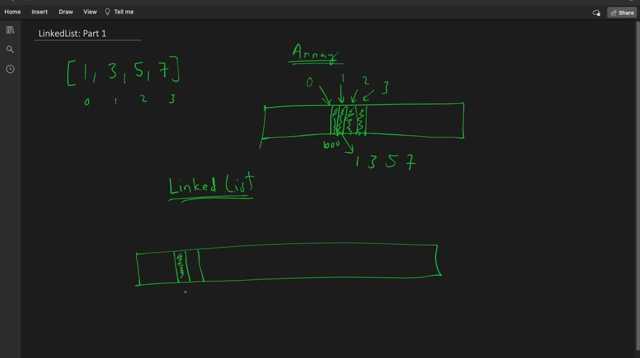 section. this is where the value is stored. 1 is stored. maybe its address is, let's say, 1000. so this is where we are starting the linked list. so start of the linked list. we have a head, so it's like a pointer, so pointer pointing to the first one. so it is like a pointer, so pointer pointing to the. 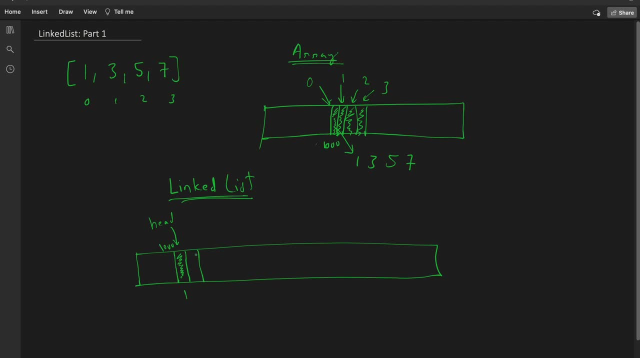 first node. okay. now their second partition is empty as of now, let's say, and so generally it has a null to indicate that the end of the node or end of the linked list. but now we have 1, 3, 5, 7, so it will store the address of some other node. so let's say, here we have our second node, okay. 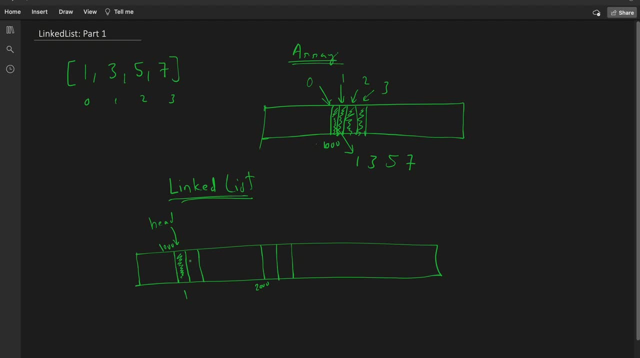 its address is two thousand. so here we will have the value 2000. so from here we can directly jump to the next node, and in this we have stored the value. that is three. again we have one more node somewhere. here we have the data. that is five. 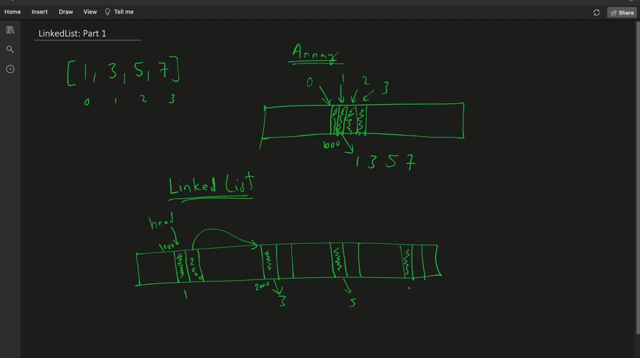 again one here. here we have the data, that is seven, but then this nodes address is, let's say, seven thousand. this nodes address is four thousand. so the previous node, this one, three, will store the value that is three, and the value of the address for the next one. so it will store four thousand. 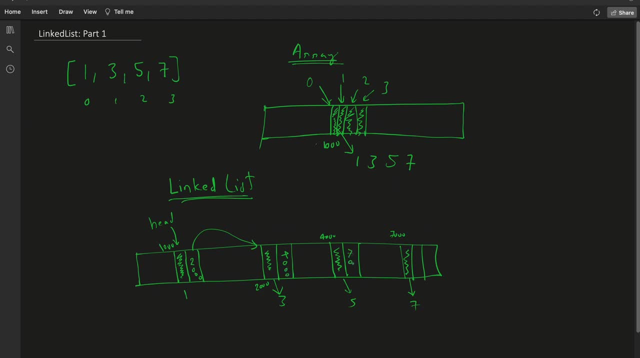 similarly, this one will store seven thousand, so this one can link us to the next node and this one can link us to the next node. now, after seven thousand, we do not have any other node. that is attached, right? so this one will have a null value. okay, this one will have a null value. 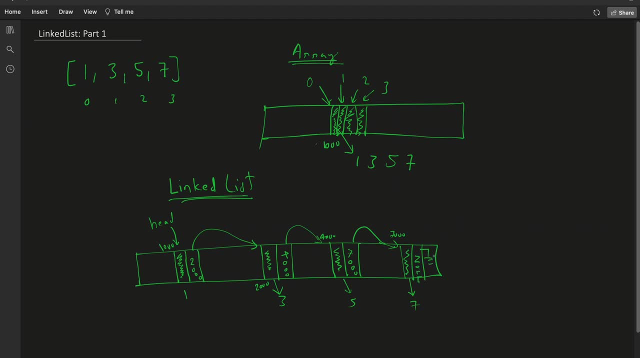 or we can do it like: okay, now what happens is if we want to insert any element after seven, let's say you want to insert an element eight, okay, what can we do? we'll create another node somewhere, maybe in this complete memory location. we created another node. node will have two. 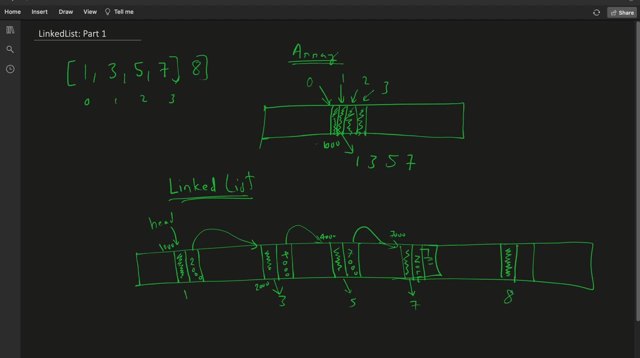 partitions one. this one will be for data, so that will have the value eight. this one is already null because only a node is created, right, but now we are adding it to this linked list. so how do we add it as part of this list completely? so this previous node seven was pointing to null. now this: 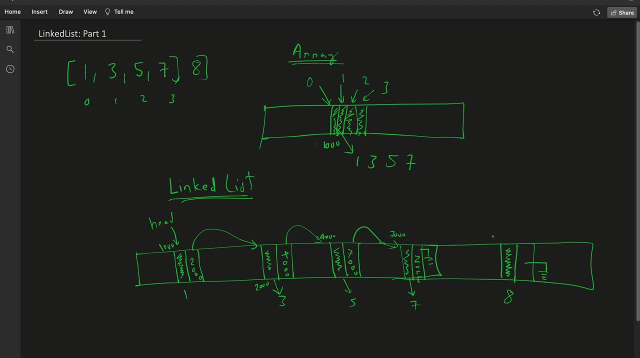 one will have the address of this node. so let's say this node has the address five thousand, so we'll put insert five thousand address here. now this can point to this node. we can get the value eight and the next is null. okay, now let's do one more thing. let's 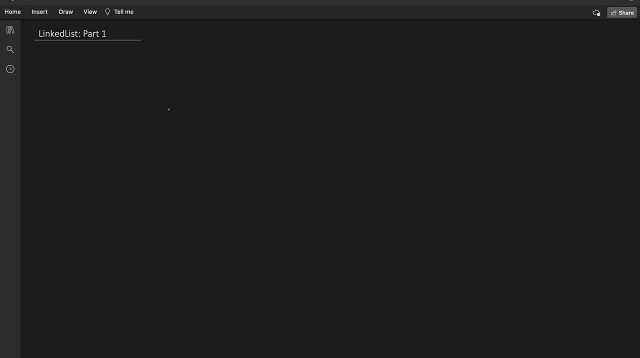 okay, now again we'll take the same example. there was one, three, five, seven. okay now, when we talk about linked list, we always discuss them like this: okay, so first we saw how they are treated in memory. now we'll see how they actually look like. okay, so we have these nodes. 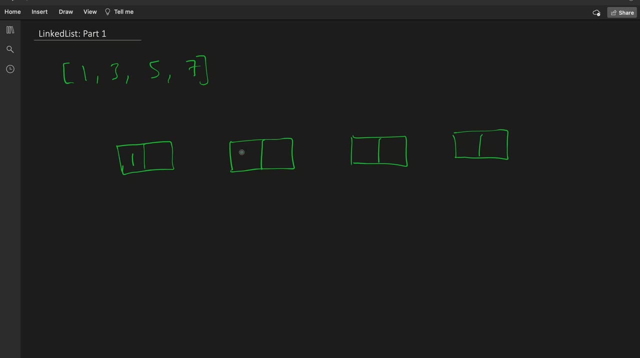 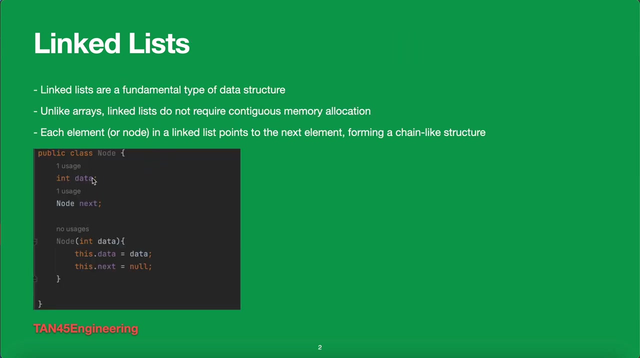 okay, so this one will have the value one, three, five, seven. this one points to the next. this is how we represent the link list. points to the next, points to the next and the last one is null. okay, if you see, here, in this example, we have seen that a node will have data and then 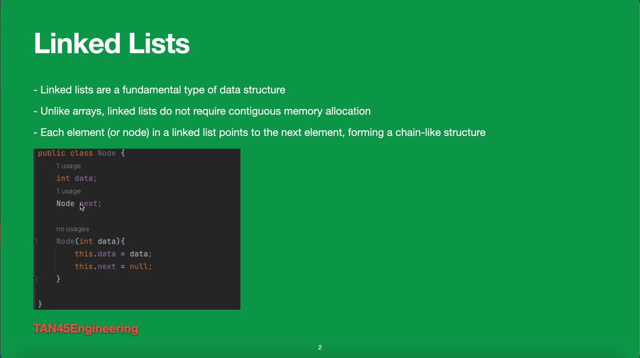 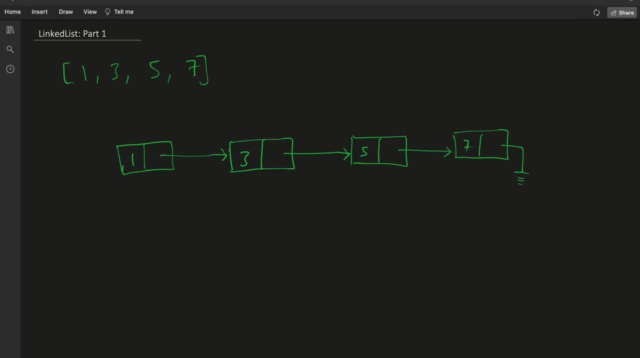 pointed to the next node, again of node type. so you can see it's a pointer to the next node, right? so we have data of integer and then pointer to the next node. as we saw in the memory, this actually has the address for the next one point dash, and from this into the next node we are creating an item, a dot. 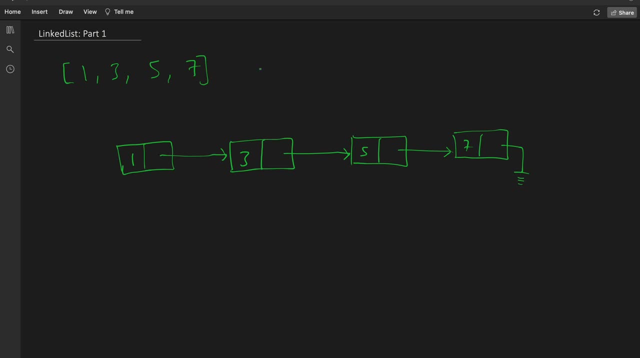 the next node. now let's imagine, and now let's compare it with an array. okay, now, before comparing it with the array, let's do how, let's see how will we traverse through this array, traverse through this list? okay, so for an array, what we were doing is we were running a for loop, okay, and then one by. 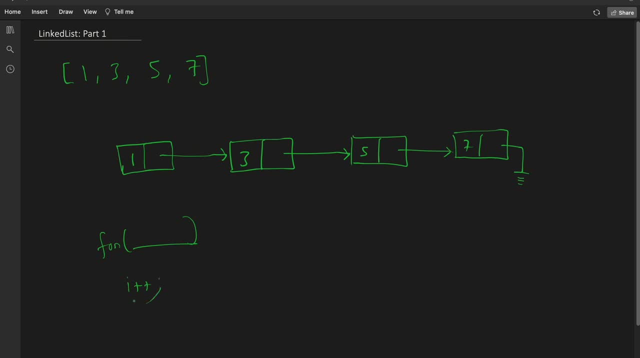 one. we were going to the next index and we were doing I plus plus, right, but in this case to. we have one starting pointer that will call it as head, pointing to the head, and we traverse this value. then we simply mark, let's say, we create another pointer- temp is equal to head, okay, so 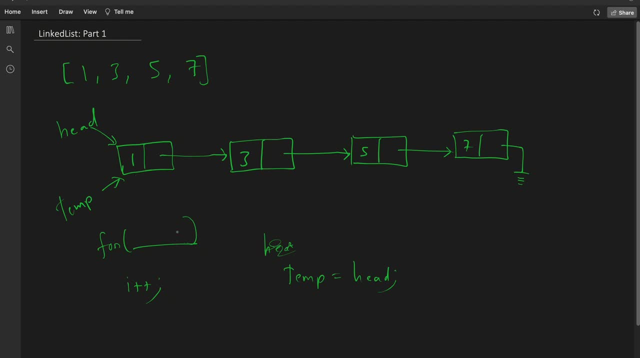 now our pointer temp is pointing to the same location where head was pointing. we can get the value like temp dot data. this will fetch us the value so we can give int a is equal to temp dot data, so we'll get the value one. then we want to move forward, so we'll say temp is equal to temp dot next. right, so now. 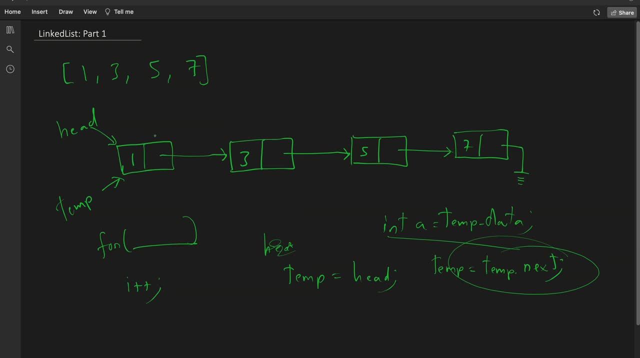 temp will point to temp dot next. this is the next, as we saw here, this is the next right, so temp will get the value of temp dot next. so now temp will point to the next because next is pointing here right. earlier head was pointing here, so temp was. 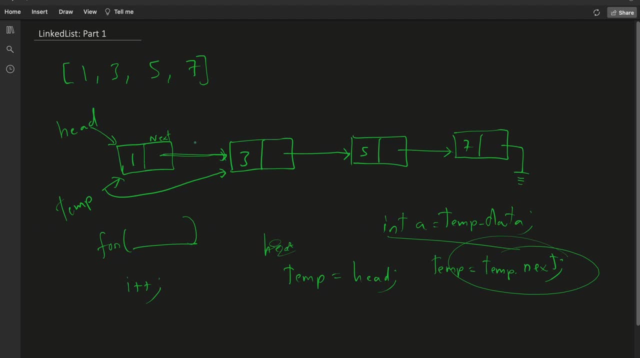 pointing. here, now we do: temp is equal to temp dot. next, temp got the value of the next pointer that is here. now again we can get the value like: into: b is equal to temp dot data. again we move forward. we do the same command: temp is equal to temp dot. next, this is: 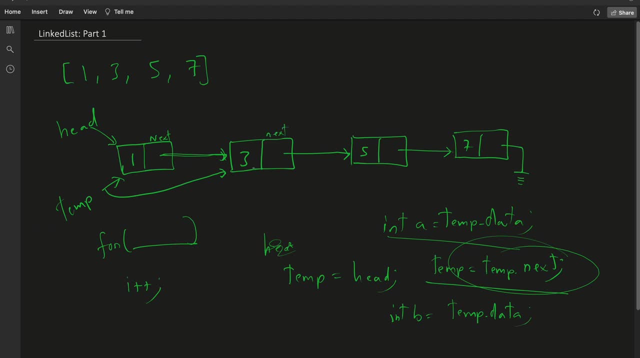 next. so temp is here. temp is equal to temp dot. next, so temp points to this one, similarly to this one. and then for a for arrays, we used to keep a loop something like this: um int. i is equal to zero, i is less than array dot length. 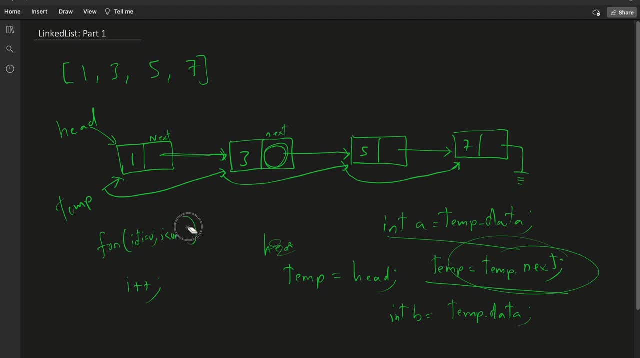 let me. let me write it a little in a little better manner. okay, for arrays, we used to do it like for int: i is equal to zero, so i would be the starting index. i is less than array dot length, i plus plus. okay, and then some code here, this initialization we are. 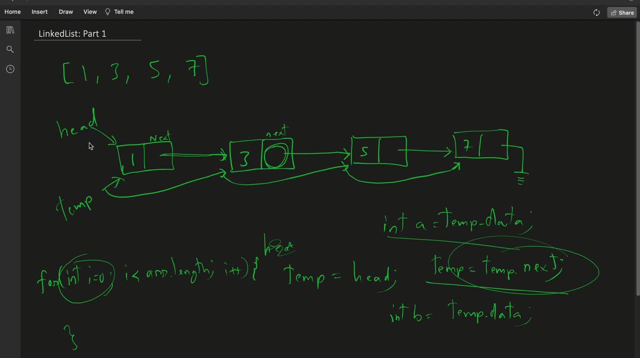 doing it with temp is equal to head. so temp gets the head. i plus plus. we are doing with temp is equal to temp. dot next, but this condition, which actually helps us in avoiding array access out of bounds. we do this by checking every time that temp is not equal to null before fetching the value, something like 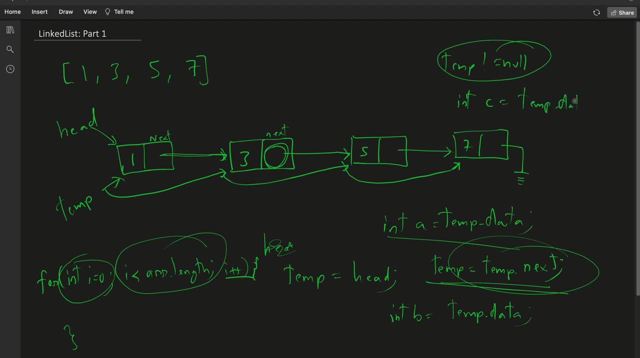 int c is equal to temp dot data. now we can add a call element here that the value can be or εί, not equal to null. then we can say: int c is equal to tempdata, So it will get the value like this. Now the question is: we used to do the same with arrays and now for this, for. 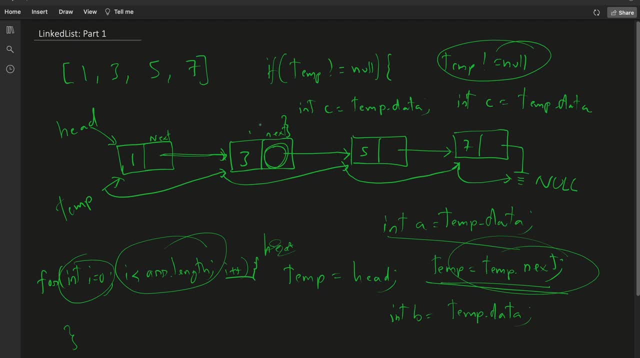 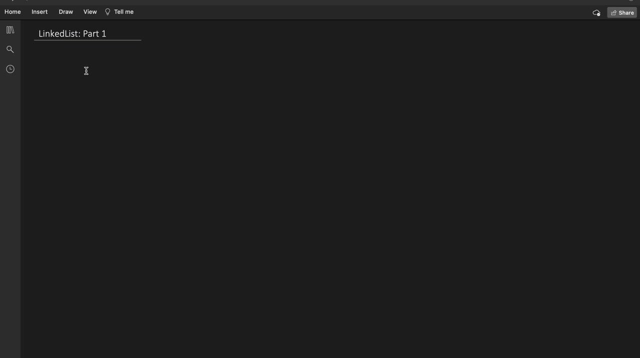 linked list also, we are using the same technique. It is slightly different, but overall principle is same. Now let's look at it one more time to understand it on a deeper level. So again we will take the same example: 1,, 3,, 5, 7.. Let's say I want to print this: 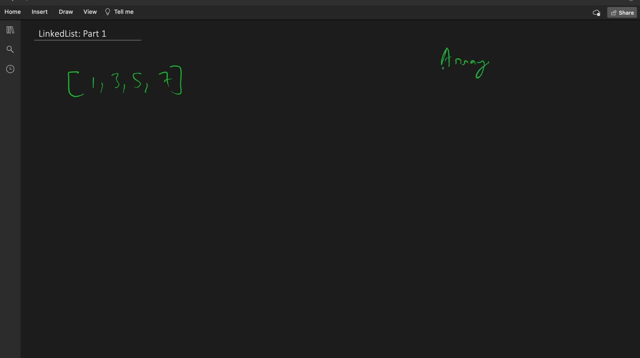 How will we print it for an array? First let's see If we were storing it for an array. we will print it something like this: For int, i is equal to 0, i is less than arraylength i++. then systemoutprintln array of i, right. 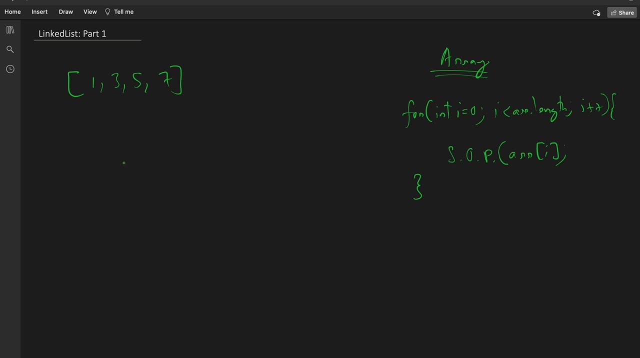 Now, how will we print for this linked list? Let's see, Let's say we have the print method print list. We could have created the same above this as well, So it doesn't make much change. Now, node- temp is equal to head. We will create. 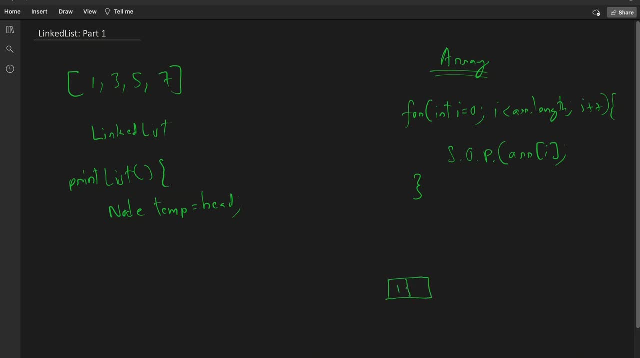 a linked list here: 1,, 3,, 4,, 5,, 6,, 7,, 8,, 9,, 10,, 11,, 12,, 13,, 14,, 15,, 16,, 17,, 18,, 19,, 20,, 21,, 22,, 23,, 23,, 24,, 24,, 25,. 26,, 27,, 28,, 29,, 20,, 22,, 24,, 25,, 27,, 28,, 30,, 39,, 40,, 31,, 32,, 33,, 34,, 35,, 36,, 37,, 38,, 39,, 41,. 42,, 42,, 34,, 41,, 42,, 45,, 37,, 42,, 46,, 37,, 48,, 49,, 40,, 42,, 42,, 44,, 45,, 46,, 47,, 48,, 49,, 44,, 49,. 501,zen, 100, 120, одна' она'ı 5 beim zit gelen. çok şekiltken başına umduhan şansımız samo, Frankان. Thank you. It was clear for most of you that this script was going to beăngı. 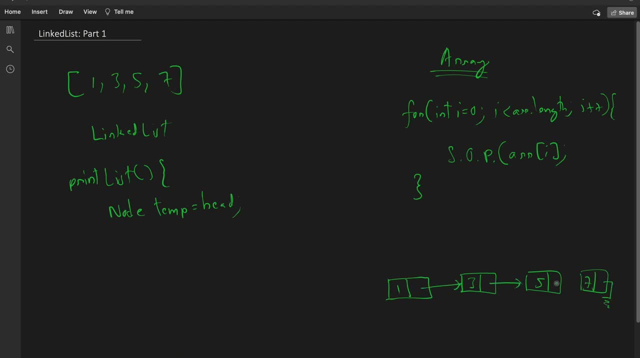 It is our home page again, thanks to the wishes of executive, So don't be beaten up. for any of you who wanted to see the top story of the days- and even if you didn't- You can submit any of it here- temp is not equal to null, because if it is equal to null, like it would happen in the last case, when 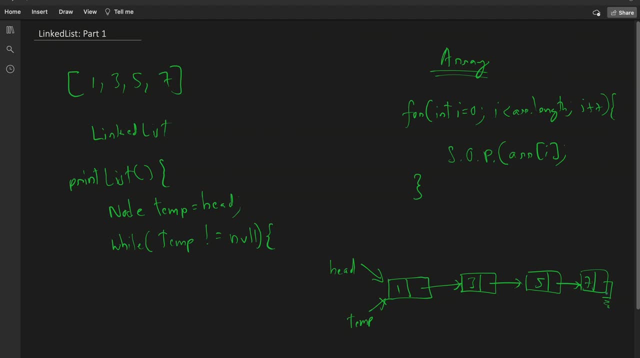 it goes to temp, dot next will reach the null in the end. that time it does not null does not have any value, right? so we do not want to say fetch the next value, so we want to avoid that. so that's why we do a temp is not equal to null. this is the same check, like this one, to keep it from. 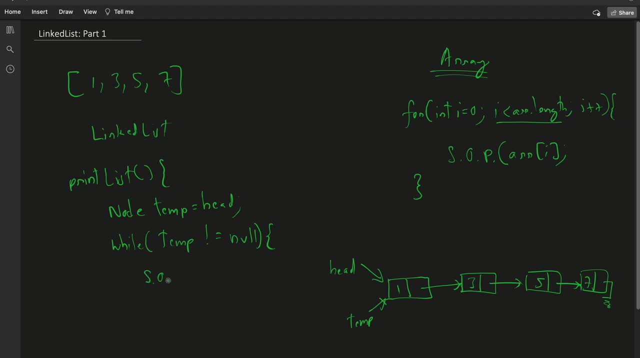 array access out amounts. so we'll say system dot out dot println and we'll print the value like temp dot data. and then what will we do? we'll move the pointer here, we'll move. we were moving the pointer using i plus plus. here we'll just say: temp is equal to temp dot. next, 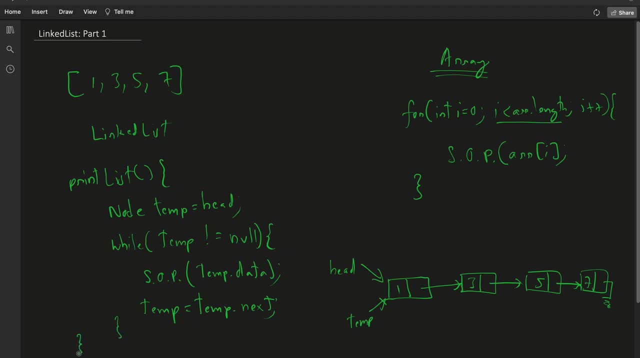 right. and this is next and this is data. so each node has uh data and next. so when we say temp dot data, it fetches the data, prints the value one. then we do: temp is equal to temp dot. next, temp moves next. then again, is temp not equal to null? uh, yes, it is not equal to null. we print temp dot data. temp dot data is. 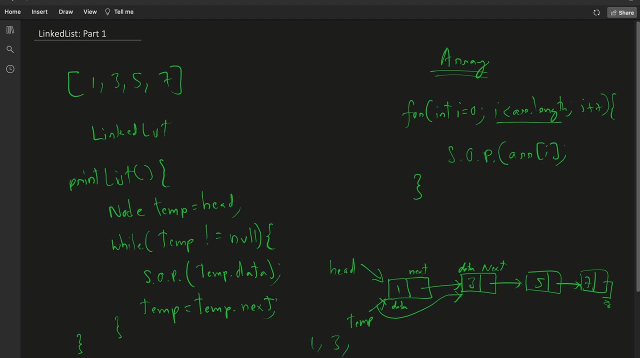 three. so first one was printed, then three was three is printed, then temp is equal to temp dot. next it moves to next, then five is printed, it moves to next, then seven is printed, then we say: temp is equal to temp dot. next it moves to next, which is null. we say: is temp not equal to null? 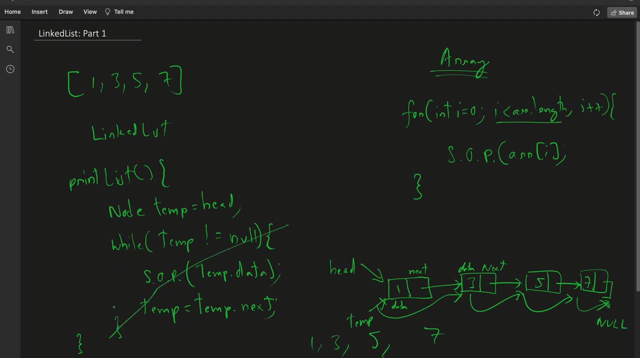 no temp is equal to null, so the loop breaks here and we come out of the loop. okay, so this is basically the linked list, or how the linked list overall works right now. let's, let's do one thing, let's discuss linked list on other levels also. okay, so we know that. as 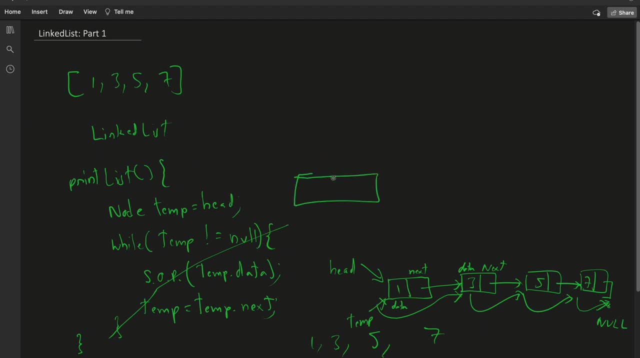 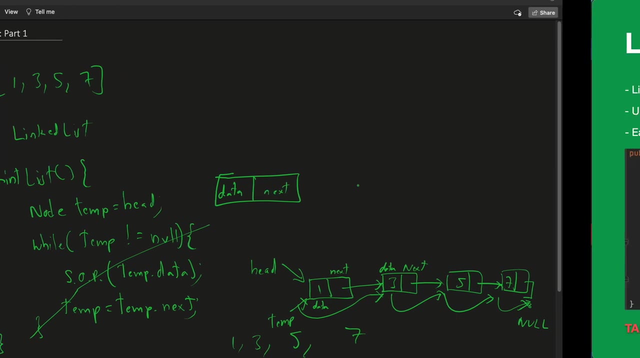 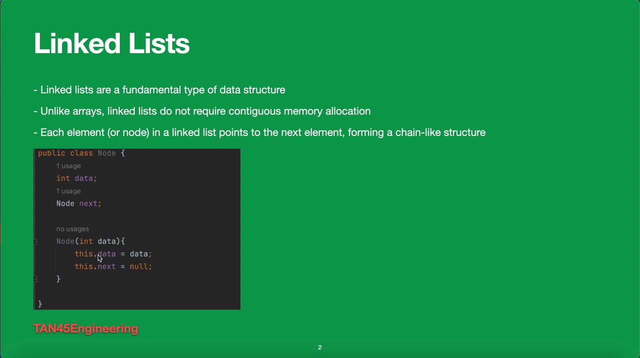 a node. this is what a node is. we have data here and we have next here, which points to the next one. okay, from the code perspective, we can see. we create a separate node, we give the data, we have the next. when we initialize another node, we just initialize the value and mark the next as 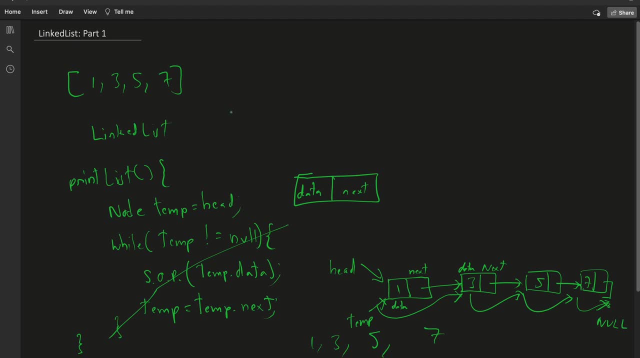 null. okay, when we connect them to the next node, that is, when we connect to that this node dot next pointer will point to the new node. okay, like one of the operations is insert, where we add one, then three, then five, then seven, so we'll do something like this: 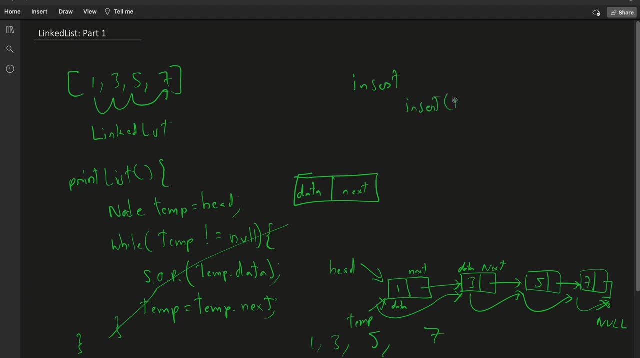 we'll say insert int data first we'll create the data. so we'll say node. now if you see node, is this node class, the node data structure, the node class. okay, we'll say node. new node is equal to new node and we'll pass the data. 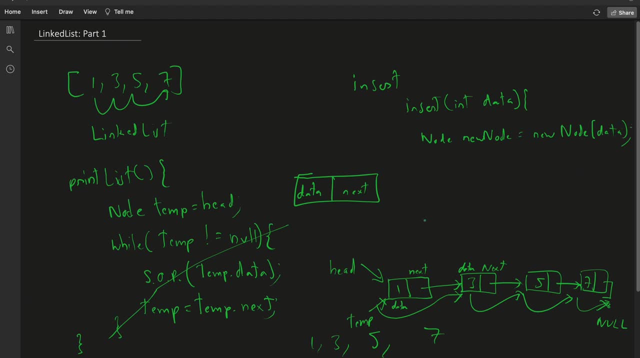 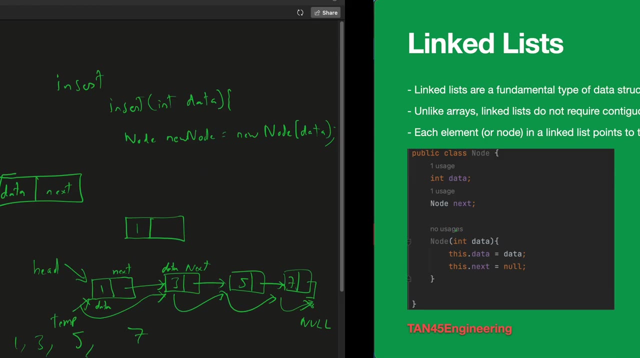 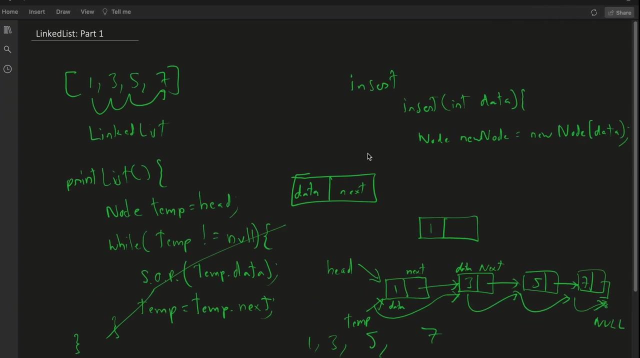 so let's say, if in the beginning one was passed, so a new node is created that has one, and what is its next point into? the next is pointing to null. this is the constructor you can see in data. this dot data is equal data. this dot x is equal to null. so it is pointing to 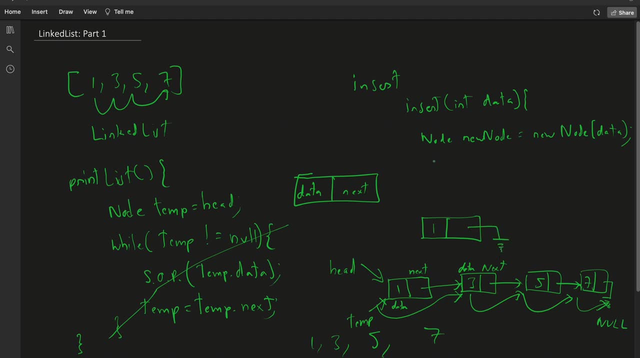 null. then we can say: node dot next is equal to head. okay. now we are saying node dot next is equal to head. so we had a head pointer. so nodes next will point to head. okay, and then we this: since this was the first value, we want the. 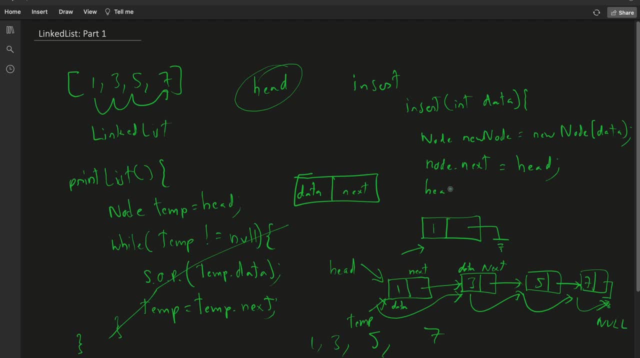 head here. so in the end we'll say head is equal to new node. now what will happen? let's delete this part. okay, so we have something like this: that we have one, the next is null and this is head. next time we insert the value three. so we int: data is equal to three, we create: node is equal to new. 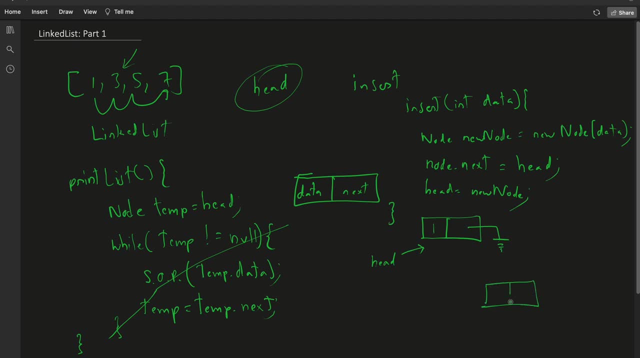 node. a new node is formed. it has the value three. the next is null. we say node dot next, so this node dot next is equal to head, right, so it's node dot next would, instead being null, it will point to head, and then head is equal to new node. so head will then point to new node. so it will become something. 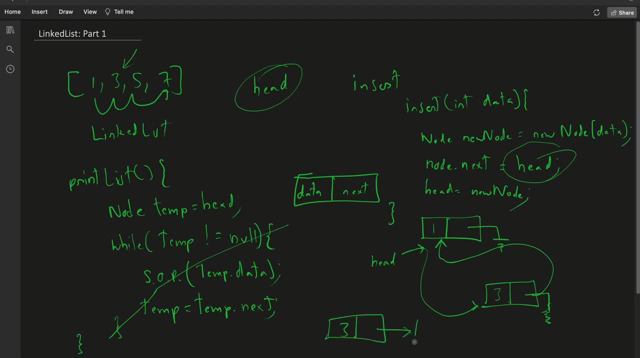 like this: three pointing to one and then one is pointing to null and head is now pointing to three. this is that we are inserting the data in the beginning. similarly, you can insert the data in the end, where each time you create another node and you say head dot next is equal to new node. so every 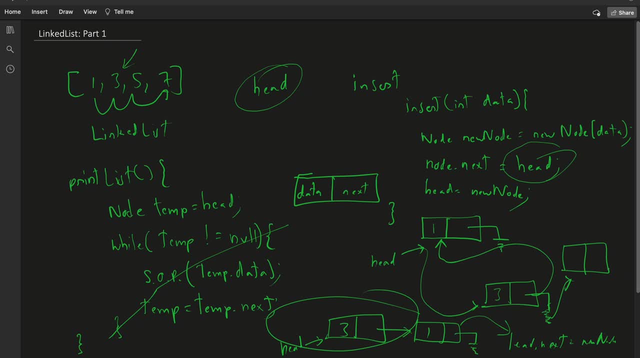 time. we'll get the next node now. or you traverse the previous node, you keep a last pointer and the next of it is the next node, or you enter them in the reverse order, so you can always create a node in the end. it will always happen like: you always create a node. there is data. this one is pointing to null. now you already 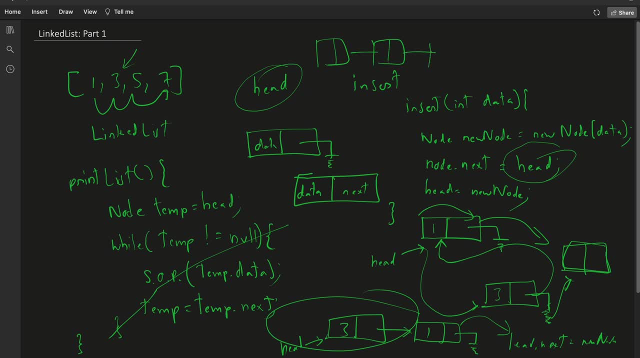 have a list that is created that is already working fine and you can directly map it anywhere. okay, if you map this data to this one, it will directly point to this one. you map this data to here, it will get inserted in the middle, so we'll come to those operations as well, okay. 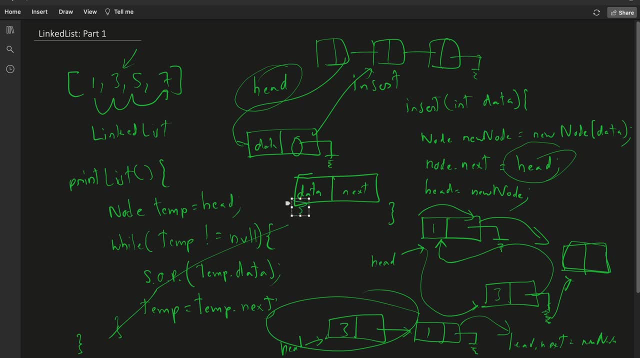 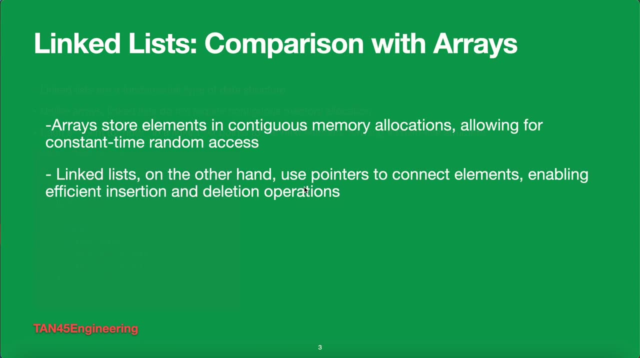 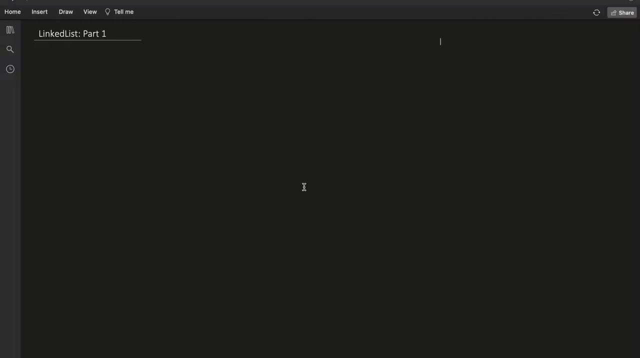 uh, okay, let's do one thing again. okay, let's move forward. so linked list use pointers to connect elements and enabling any efficient insertion and deletion operations. okay, let's look at the insertion and deletion operations on linked list and arrays. so we have one, three, five, seven and we want to insert the. 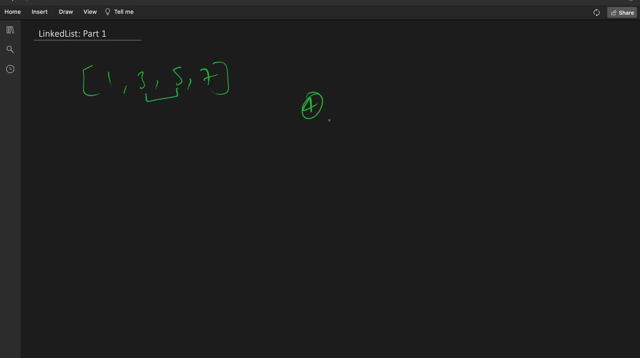 value four in the middle of this. now, how will it happen? for arrays first, let's discuss for arrays. now, arrays in memory. they are stored in contiguous memory location. okay, one, two, three, four. so we had only four slots here. now you want to insert four in the middle, right? so what do we do? we create another array of size. 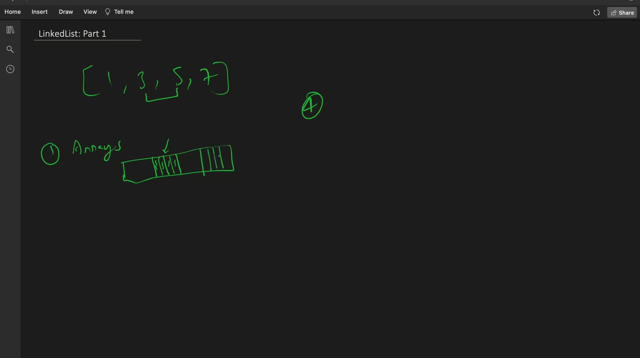 five, one, two, three, one, two, three, four, five, and then we insert one by one. we insert one, then three, then four, then five, then seven, okay, if you see? see, this is very tedious process. so you have to create new array with new size and then previous array will be deleted. previous array will be deleted, okay, so 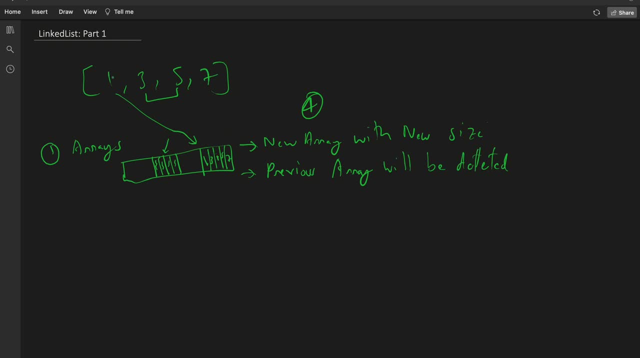 if you see, insertion is quite difficult here. of course, fetching the elements, getting the elements is easy for arrays, for linked lists it's difficult. we have the for linked lists. the only possible way is to traverse. so we have 1, 3, 5, 7 and I. 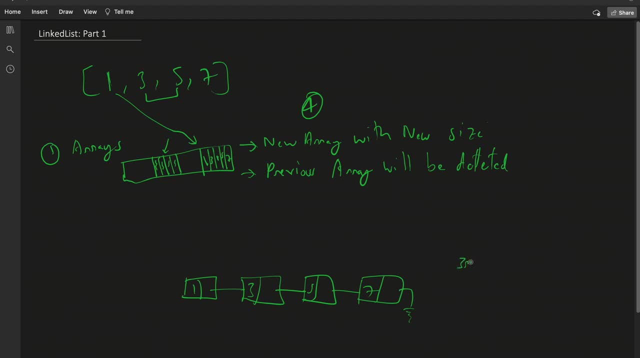 want to find out the third element, So I have to go one by one. I go to one. I keep a counter. this is my first element, then go next. this is my second element, then go next. this is my third element. I print. 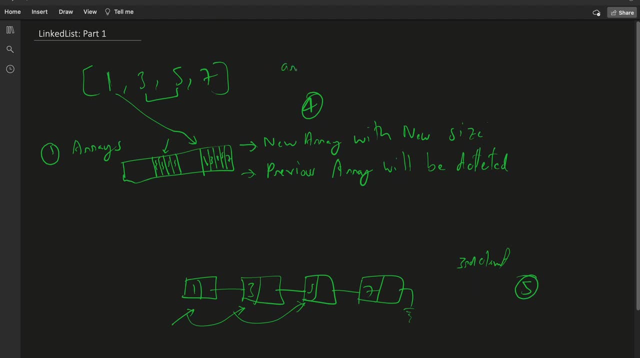 five Here for arrays. if I want the third element I can directly say array of two. that's it. But for insertion it is very difficult to insert in arrays. but how will it happen for a linked list? Let's see how will it happen for linked list. 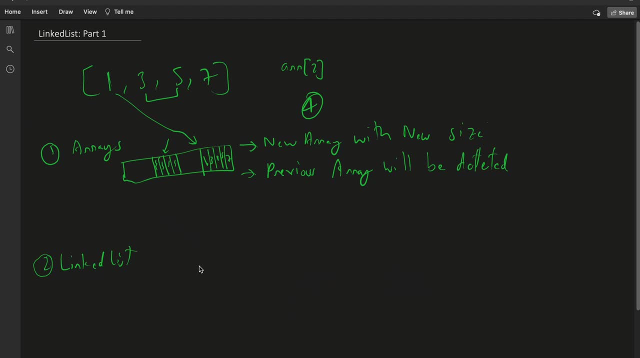 And this is one of the very famous reason why we have the linked list data structure. So for linked list, we had one, we had three, we had five and we had six, Seven, five is pointing to seven, three is pointing to five, one is pointing to three. 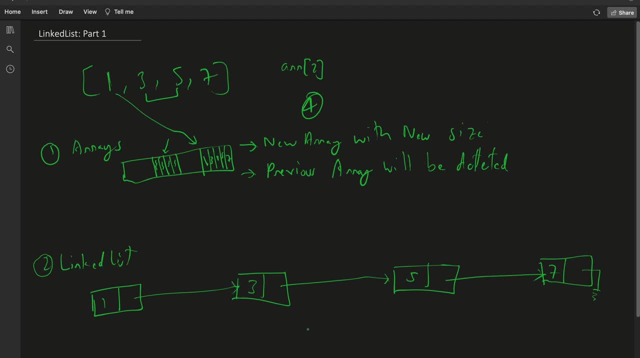 Now we want to insert four in the middle of three and five. So we'll create another node, four. another node is created, simple, we'll say four should point to the next of three. So whatever three was pointing to Four dot next would be three dot next. 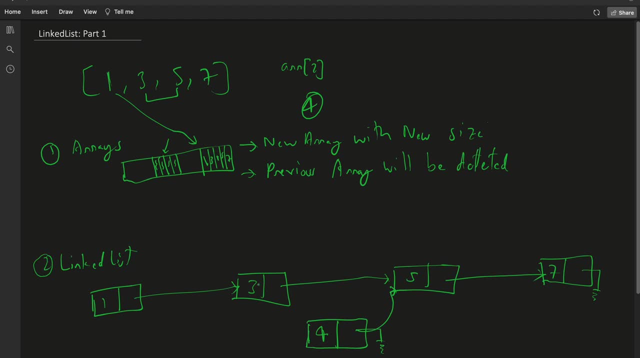 So this will point to five and will point three's next pointer to point to four. simple, We didn't have to break the list, we didn't have to create new one plus in memory, if you see, let's say, one was stored here with this address. the next pointer, three, was: 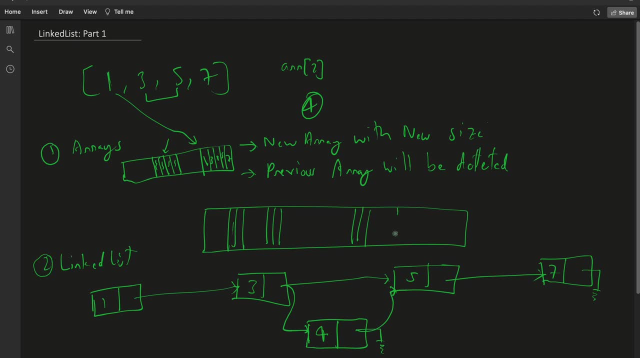 stored here. five was stored here, seven was stored here. Now four is created here. we are just seeing one points to three, three points to four, four points to five, five points to six, five points to seven and seven points to null. 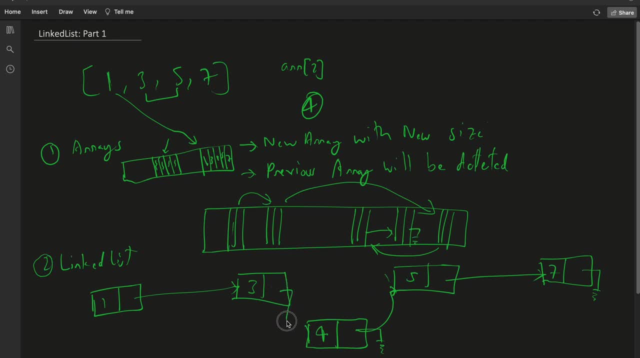 So what will happen? this path will get deleted and three will point to four. this will get deleted. four will point to five, five will point to seven. So insertion was very simple for linked list in comparison to arrays. Similarly, deletion. 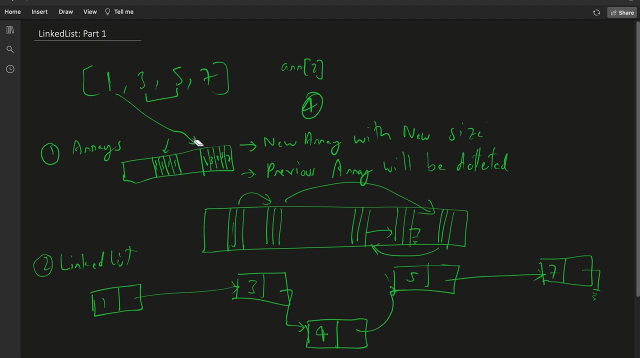 Now let's say we want to delete- Okay, We want to delete three. So what will we do for arrays? we will create another array. we will create another array in the memory location of new size, that is, three. then we will store one, five and seven. 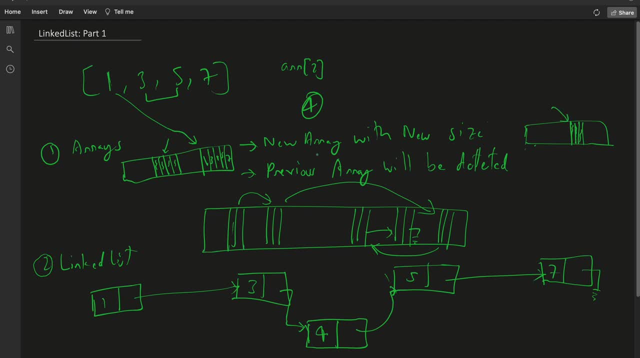 What will we do in case of so? again, this operation would require new array with new size and then previous array getting deleted on its own. Can I get it back? oh no, okay, I'll create it again. this was three. this is pointing. 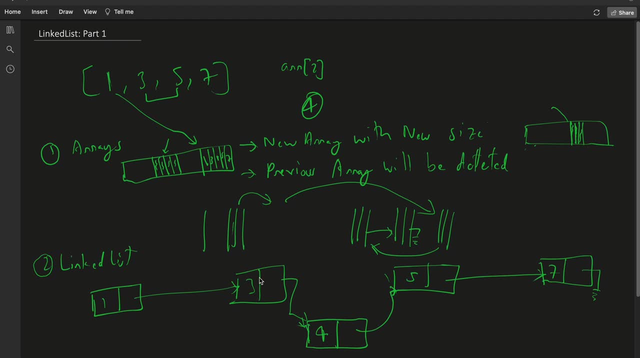 here. Okay. Now, in this case, if you want to remove three now- let's imagine this is not there- okay, three was pointing to five. Now we want to remove three. what will we do? one will directly point to five and then. 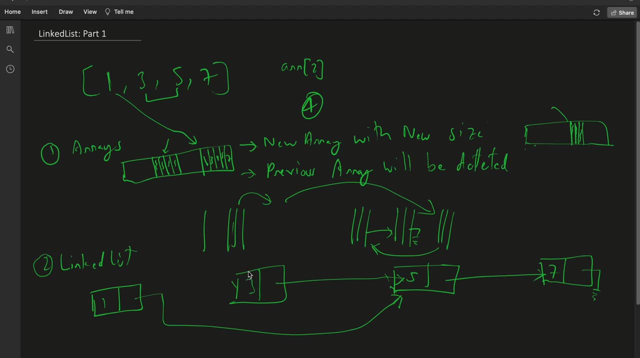 since there is no pointer pointing towards three in the end three will get garbage collected, So three will automatically get removed and one is directly pointing to five. So it was very easy for linked list. So insertion and deletions are very easy. operations with linked list in comparison to arrays. 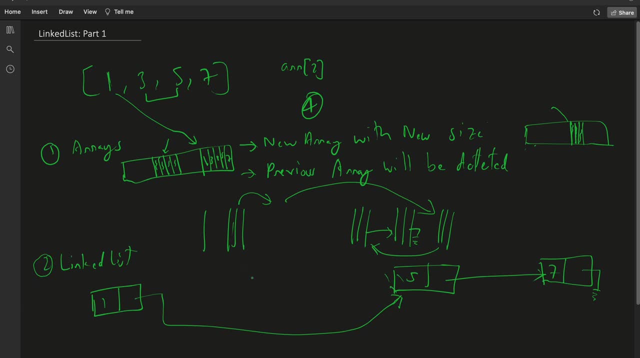 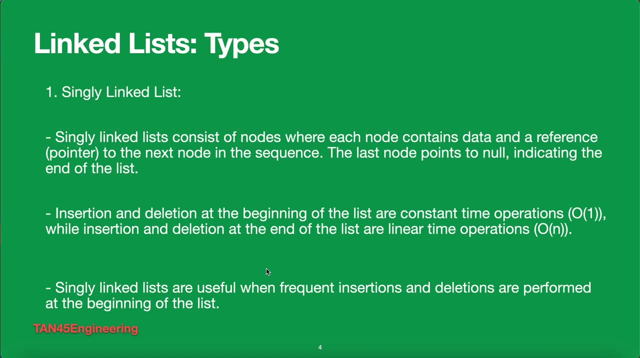 Searching of elements is very easy in arrays in comparison to linked list. Okay, With this, let's move forward. Okay Now, when we discuss linked list, there are several types of linked list. So one is singly linked list. Singly linked list consists of nodes, where each node contains data and a reference to. 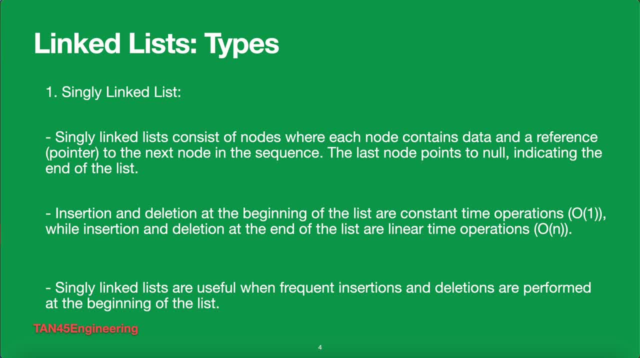 the next node, The one that we have been seeing right now in all of our examples. So, okay, let's just go through the types and then we'll understand them with the approach. So insertion and deletion at the beginning of the list are constant time operations. O. 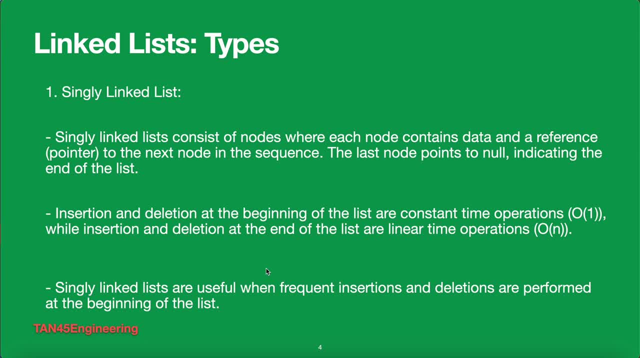 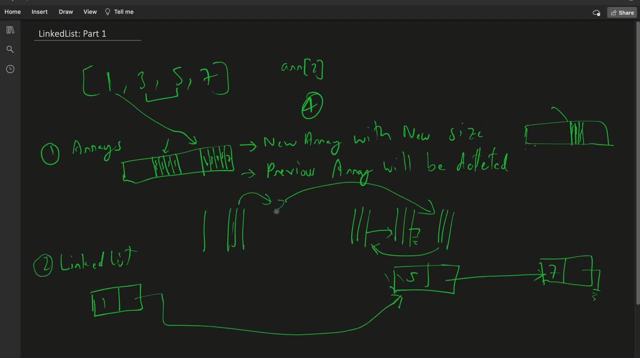 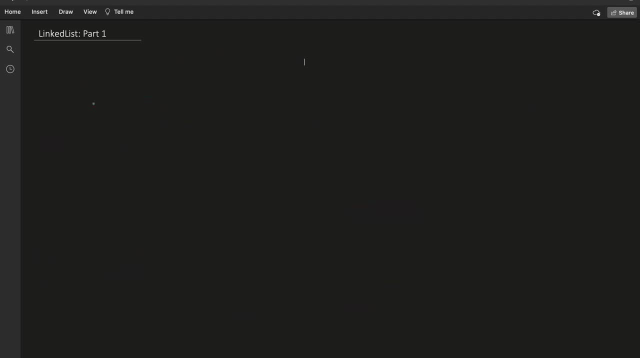 of one, while insertion and deletion at the end of the linked list are lenient. Okay, I'm not sure if you guys are familiar with time complexity and space complexity, but I'll make another video on that one, But for now let's understand. 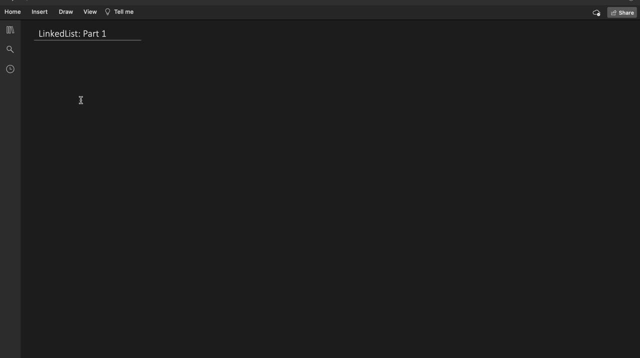 So we have this link. We have this. Why is it not typing: Okay, We have this linked list. right, We have one. I'll write it: One, three, five, seven, Pointing to five. Okay, We have this linked list. 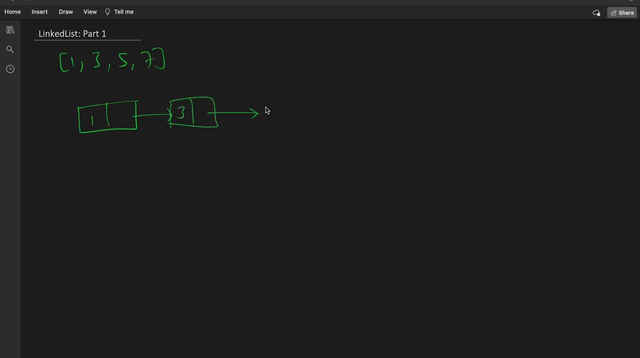 Right, We have one, One, two, three, pointing to five, pointing to seven. So this is singly linked list. It starts with a head and set a null So you can start. you can go forward as long as you do not detect a null. 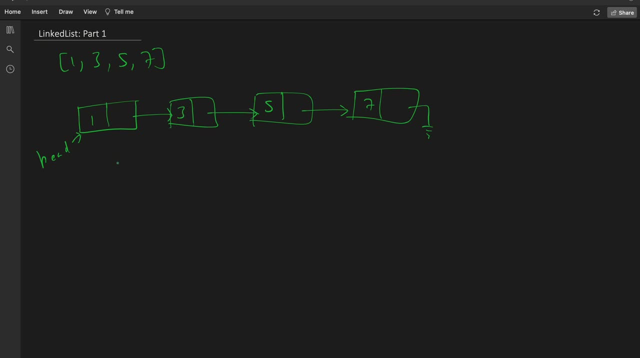 And that's why it's a singly linked list If you want to add any node to it, as we discussed, we add a node, new node. Let's say zero and I'll mark zero, dot next. So this new node, dot next, is equal to head. 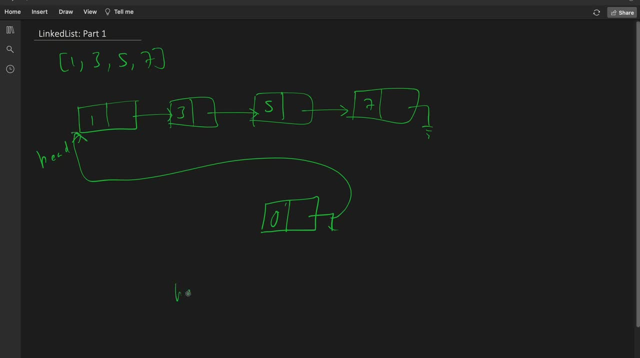 So this will point to head, And I will say head is equal to new node, as you saw in the examples earlier. So now this will become our head and a new list will become zero, one, three, five, seven. Similarly, if I have to delete, 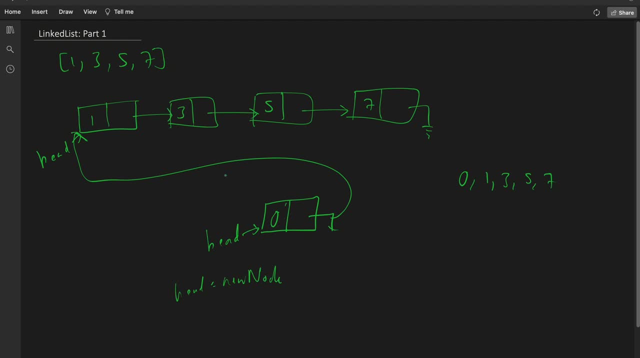 Okay, Okay, Okay, In the beginning of the list. So adding at the beginning of the list or deleting at the beginning of the list. for deleting I'll simply say: head is equal to head dot next. So head will directly point here. 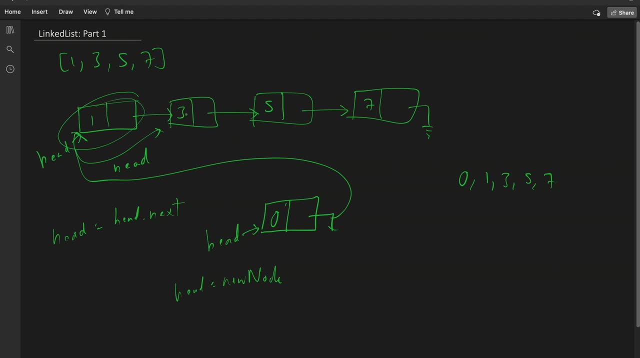 So this will become a new head. This one will automatically get out of the list. So we'll have the new list here as three, five, seven. So it's a very easy right. It's in the beginning, So it's a constant time approach. 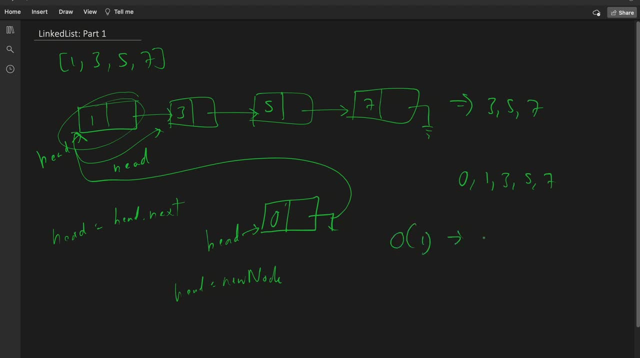 So it's O of one time complexity that is constant. Every time it will take the same amount of time. But imagine that we have to insert a new node at the end of the linked list. Okay, So, So, So So. 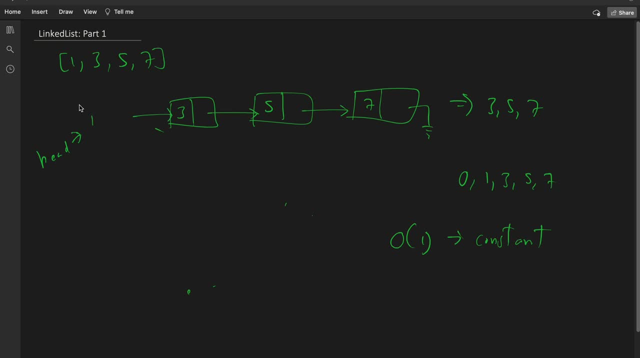 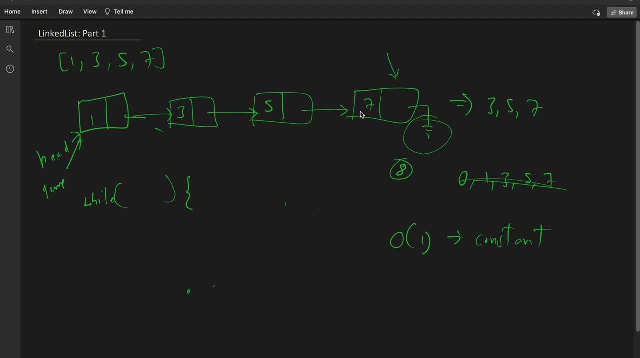 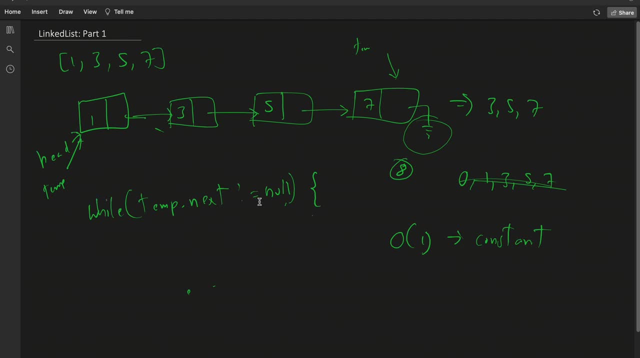 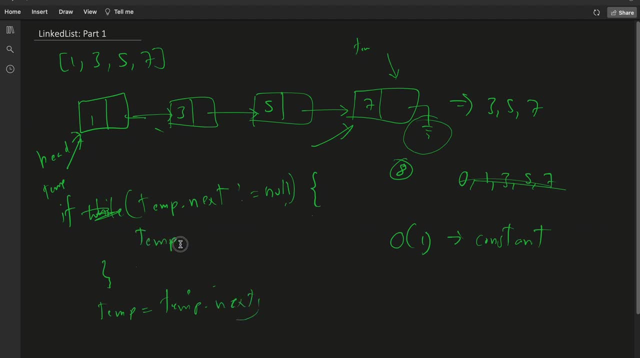 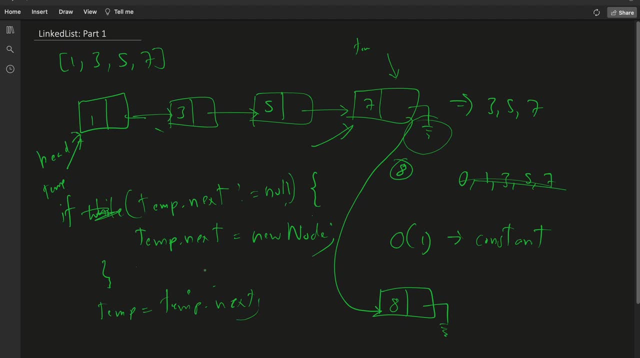 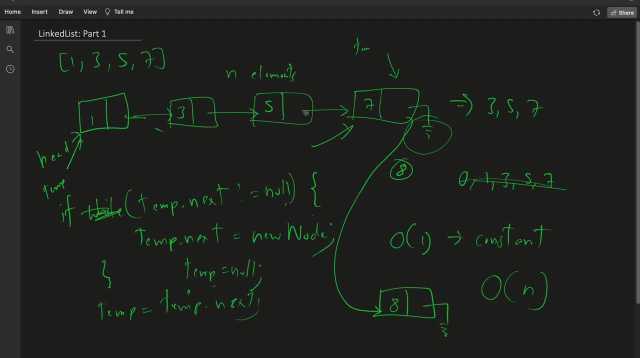 temp is equal to null, so we'll mark this as null. okay, so so next of the previous node, equal to null. but again, in this also we have to traverse the complete list, right. so insertion in the beginning of the list on the head or deletion in the beginning of the head list is: 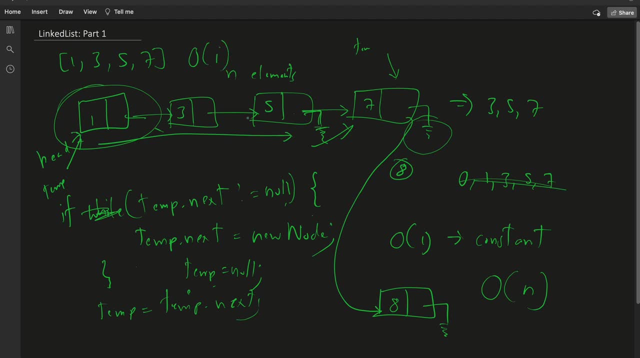 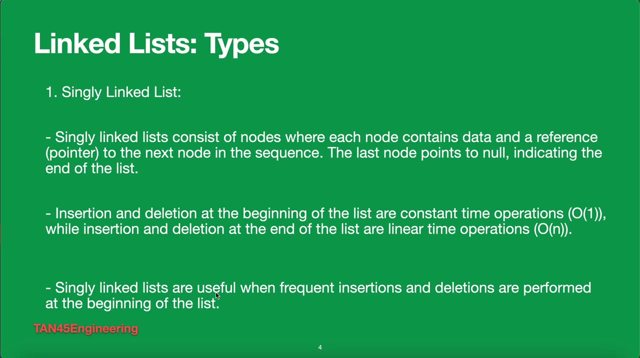 constant time, that is o of 1, but insertion and deletion at the end of the list is o of n time. complexity- okay, let's move forward. and this is singly linked list. okay, singly linked lists are useful when frequent insertions and deletions are performed at the beginning of the list. 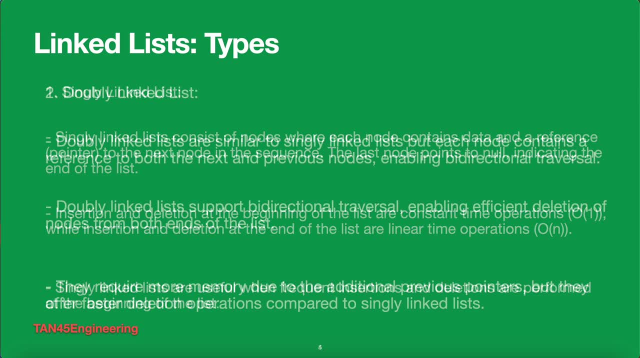 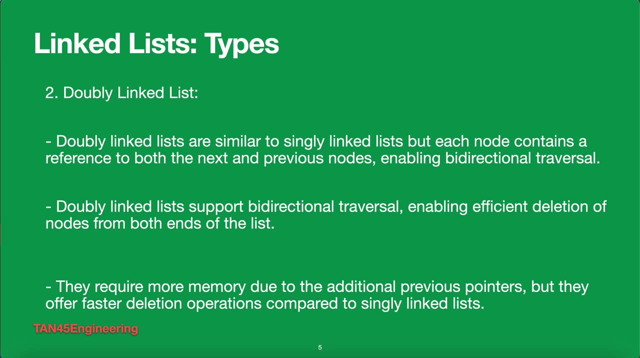 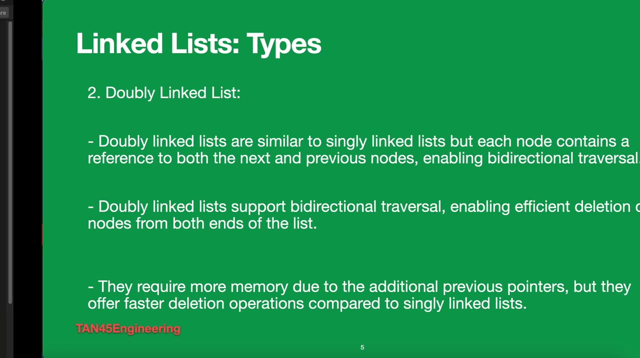 that is understood right, let's move forward. uh, second type is doubly linked list. so doubly linked lists are similar to singly linked lists, but each node contains a reference to both the next and the previous nodes, enabling us with bidirectional traversal. okay, so to understand the example here, 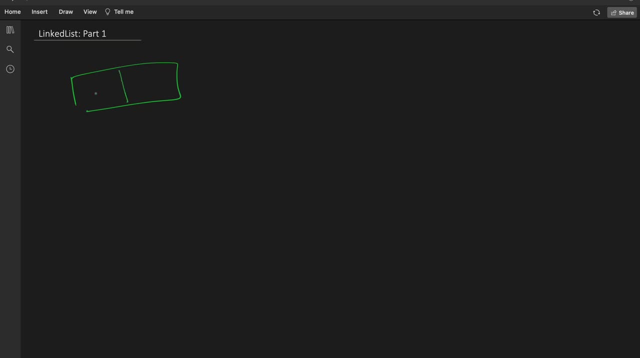 okay, this was singly linked list. okay, linked list where we have data and pointer to next. now in doubly linked list we have something like this: we have the data in the middle, we have two pointers: one is to the previous and one is to the next. so if we have a list something like this, one, three, five, 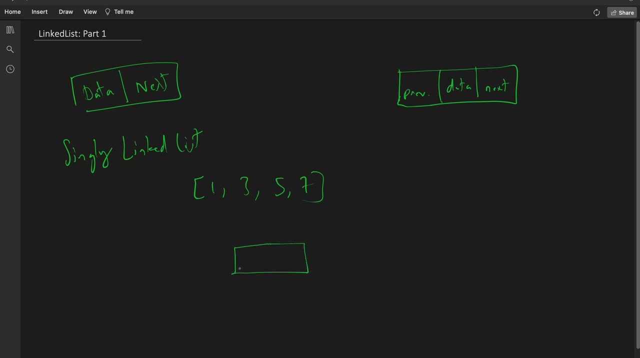 seven. we will have something like this one now let me create it here. okay, so we will have one: three, five, seven. the next of seven is null. the previous will point to five. five, five's next points to seven. five's previous points to three. three's next points to five. 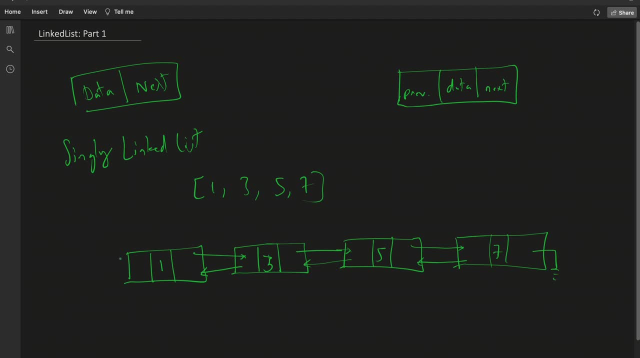 one's next points to three, three's previous points to one, and this is head, and previous of this is null. okay, now, this is what happens with a doubly linked list. doubly linked list, we can traverse in either direction. so let's say we are at the node, we are given the node. 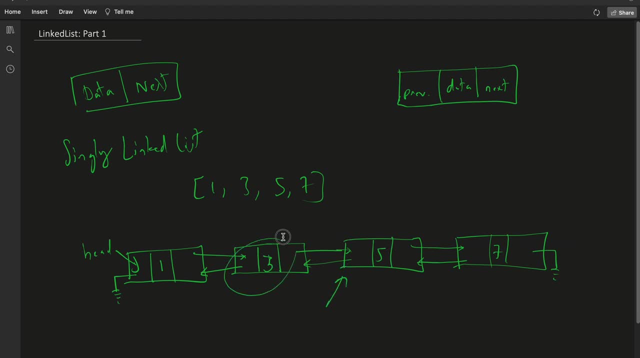 five, we can check directly which is the previous element and similarly we can check which is the next element. this is generally helpful. let's say you have a question something like this, that delete element or delete node previous to five. so what will you do in this case? for? 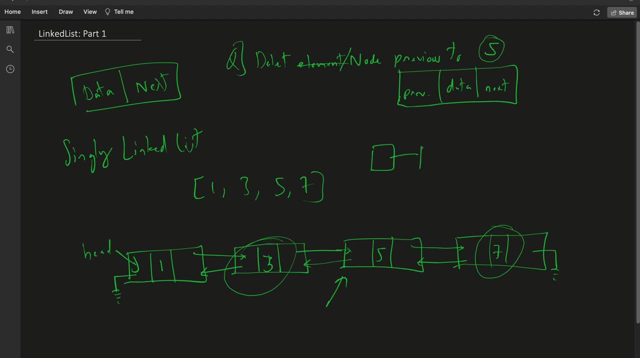 a singly linked list for a singly linked list. we have this approach right. we want to delete three, but how will we delete? we start the traversal from one. we- the question says- delete the node previous to five. then we go to three, but we still don't know that we have to delete three. then we go to five and now we know that we. 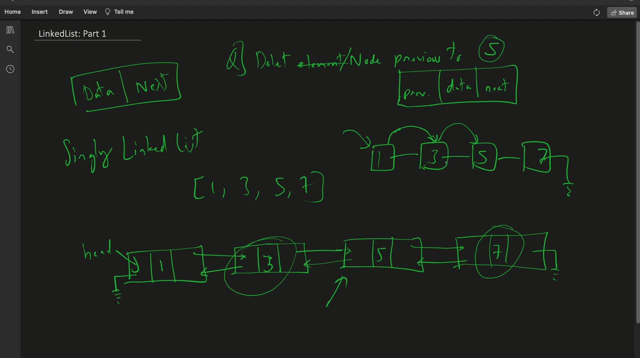 are supposed to delete the previous node right. so this this makes it easy, so we can do it. it difficult for us because we cannot jump from 5 to 3. there could, we could have used several approaches, like keeping counter like at 1, the counter was 1 at 3, the counter was 2 at 5. the 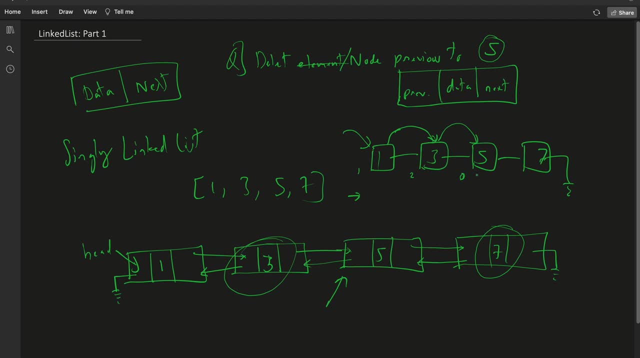 counter was 3. so we do a traversal again. and now, since the counter is 3, we have to delete a counter minus 1 node. so next time we come 1, we come 3, counter is 2, we delete this node, right. but again, while deleting this node, what do we want? we know we need a pointer to the previous node to point. 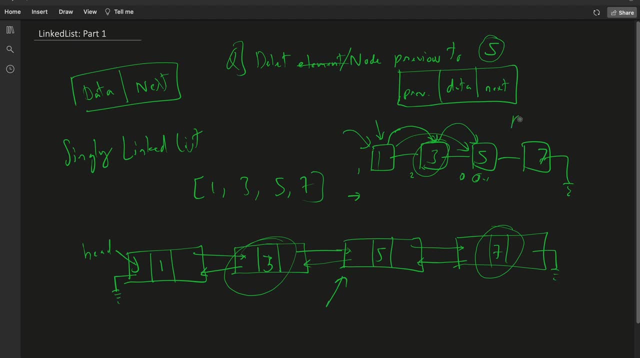 it to the next node, right. so we have to store it separately, creating another pointer, and at each state we update the previous pointer as well. similarly, other approach is directly that from the beginning you keep a previous pointer, let's say previous pointer- you are keeping as temp the next. 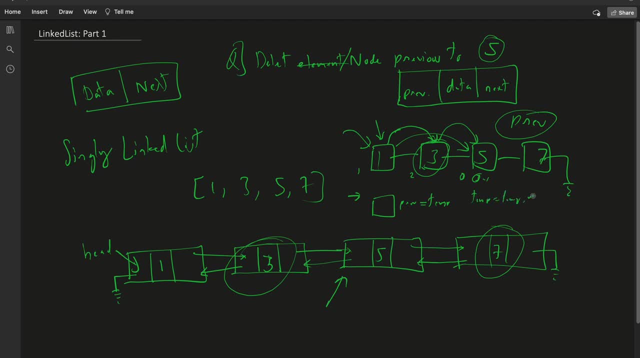 moves to temp is equal to temp dot next. so temp keeps moving and the previous one is still pointing to the last temp. when the temp moves to 5, previous would move to 3 and then when you get the value 5, you can say from the previous one that we can delete. 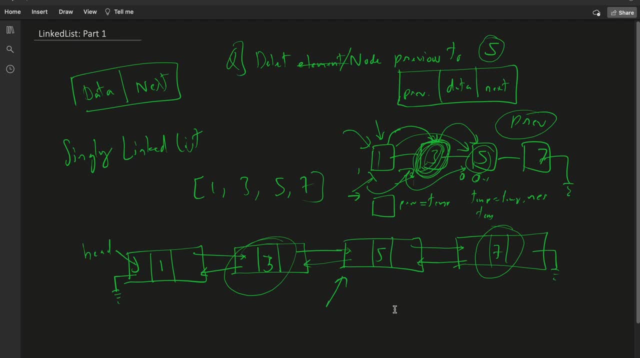 this one. but it's much easier when you have a w linked list, because with w linked list you go 1, you go to 3, you go to 5. okay, you got 5. we want to delete the previous node. so what will we do? we'll say 5, like this: 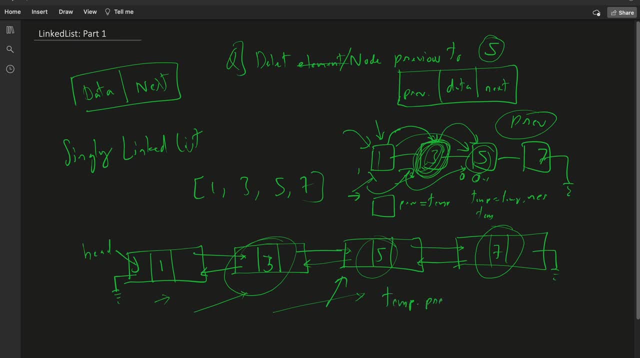 let's consider w is equal to 5 and we have all this. begin with this node. let's say this node is temp, temp dot previous. so temp dot previous is equal to tempprevious previous. so we are saying tempprevious should point to previous dot previous, and then temp dot previous dot previousnext. 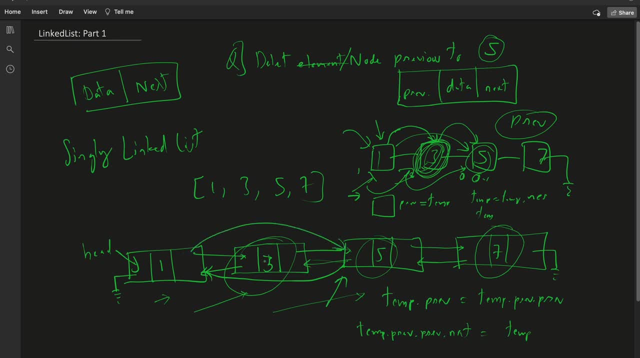 next should be temp, so we can directly change the pointer to point from 1 to 5, and from 5 to 1 and 3 will get out of the list right. so this is one of the benefits for doubly linked list and this is how a doubly linked list is made one. 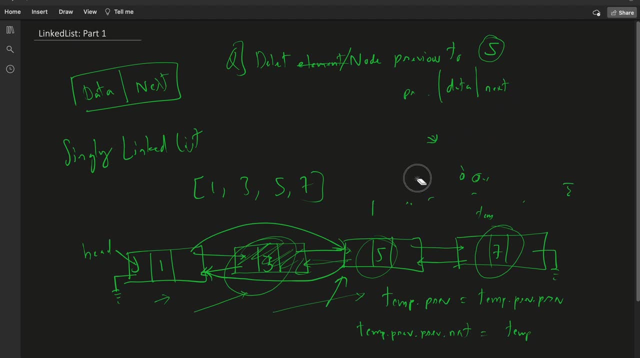 more thing: if we, when we declare the class for the node for doubly linked list, like we were doing it for a singly linked list, we will do it something like this, where we create a node class and we say int data, then we have node previous and node next. 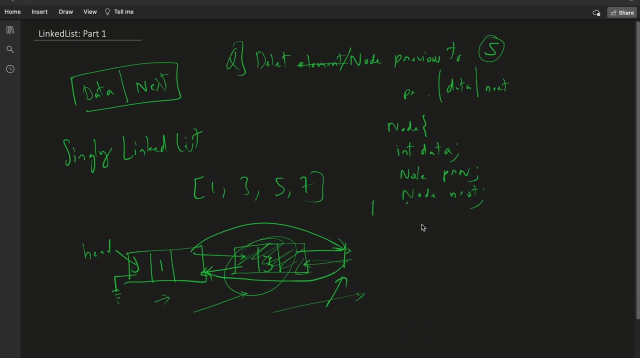 and similarly we will have our constructor node, int data. what will we do? this dot data is equal to data and previous is equal to next is equal to null. okay for singly linked list. we didn't have the previous pointer here, so we didn't need it here. for w linked list, we have the previous pointer and the next pointer. 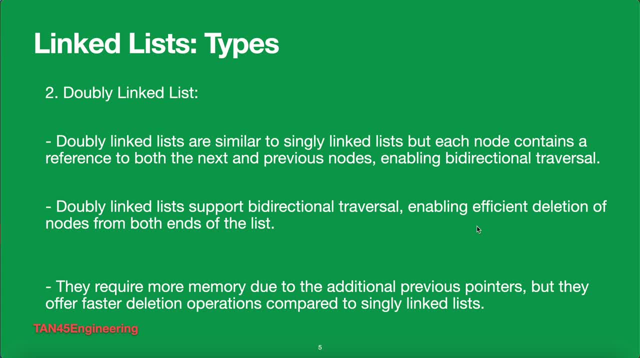 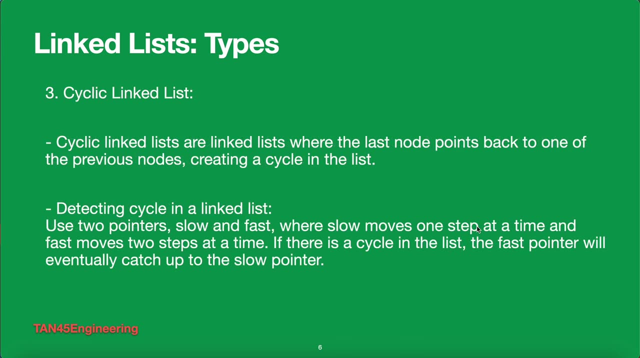 okay, let's move forward. uh, also, the w linked lists require more memory due to their additional requirement for saving the pointer to the previous node as well. right, uh, third type of linked list is the cyclic linked list. okay, so it happens when you have a circular linked list. okay, cyclic lists are linked list where the last node points back to the one of. 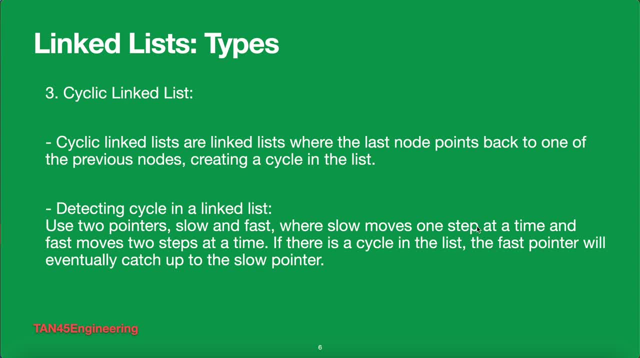 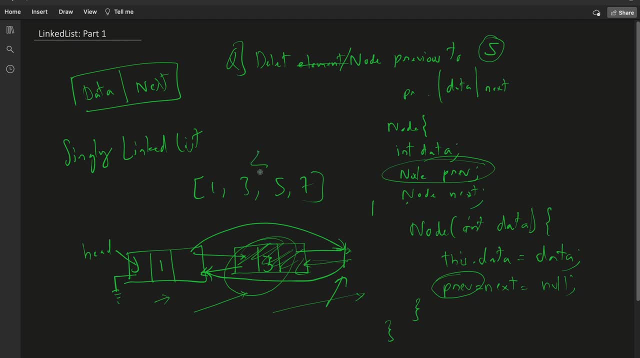 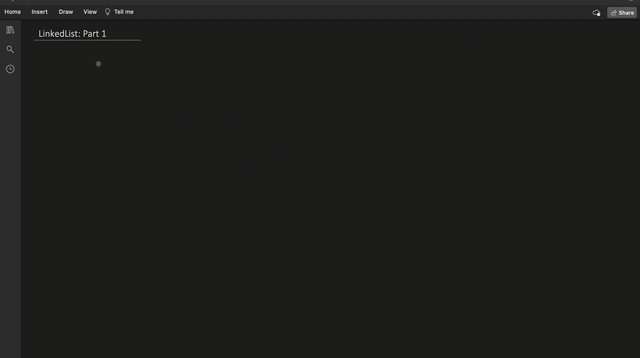 the previous nodes, creating a cycle in the list. so it says one of the previous nodes. it need not be the head node again. okay, let's quickly look at the example. uh, so i'll say command d delete. okay, so we have one, three, five, seven. okay, let's see. 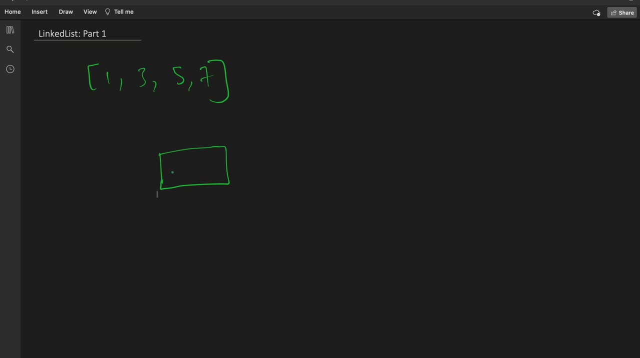 cyclic linked list can be in singly linked list or doubly linked list. okay, so we'll say singly linked list. we have one, it points to three, which points to five, that points to seven, and for singly linked list this was used to be null right, like this, but 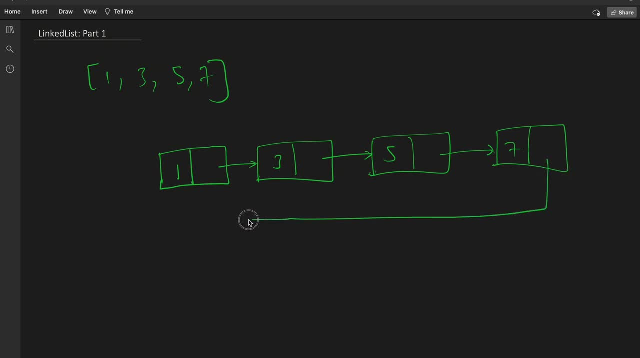 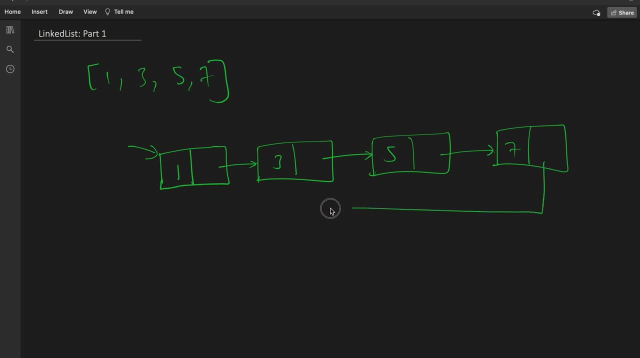 also, it can happen that maybe this points back to three or it points back to five, but in either case we do not have a null pointer here. so once we come into the cyclic loop and we go with uh, traversal while temp is not equal to null, we are saying temp is equal to temp, dot next. 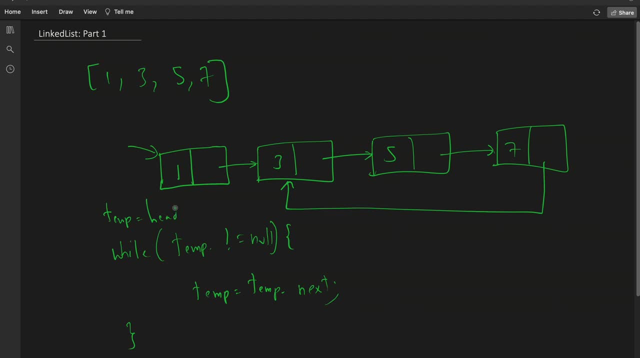 and temp was initially initialized to head, so this is head. we created another pointer, temp. now temp points to head, so temp is pointing here. so temp is not equal to null, temp is equal to temp dot. next temp came here. not equal to null, temp is equal to temp. next, then five, then seven. after seven, back to three, then five. 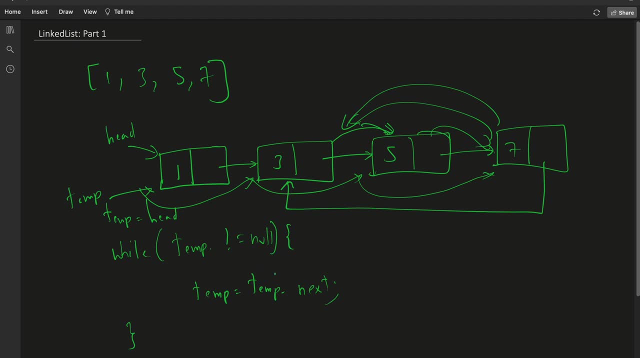 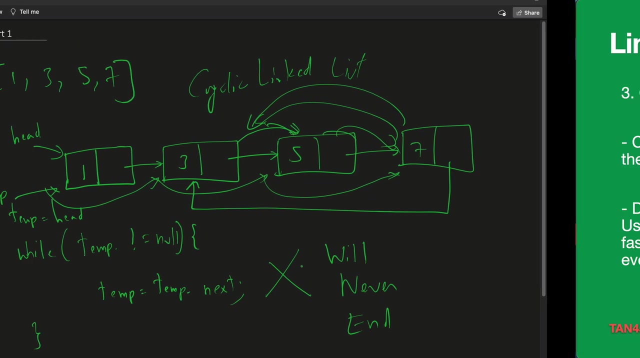 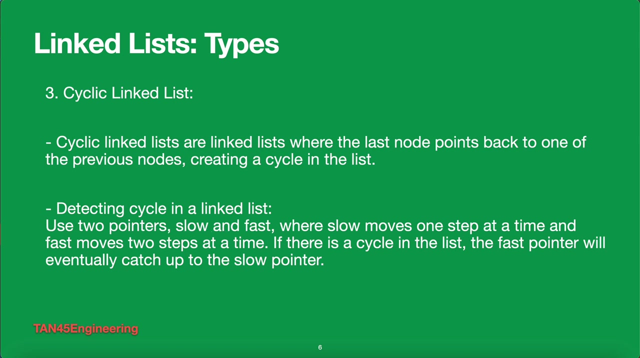 then seven, then three, then five, then seven, so this loop will never end, will never end. so now let's move to the next step, which is a link list. so this is an example of cyclic link list. okay, now let's move forward. uh, detecting cycle in a link list. so this is one of the most common interview question. plus, it is: 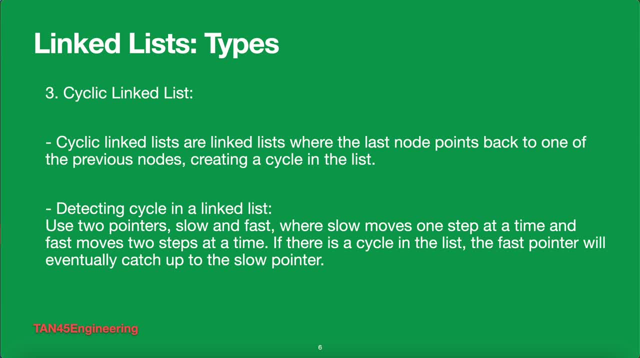 asked a lot of times- whenever we discuss linked list or whenever we discuss cyclic linked list. so can use a two pointer approach where you have a fast pointer and a slow pointer and if there is a cycle they will always catch up on the same node. we will be discussing them in the 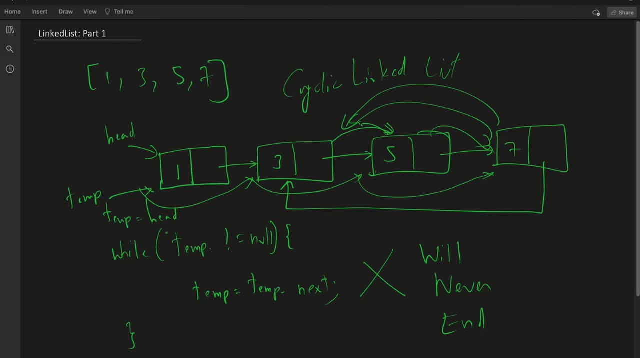 part two with code examples. but for understanding, it's something like this: let's say: let's consider this example only. okay, so we have one, it points to three, it points to five, it points to seven and seven then points back to three. so what we'll do is we'll create two pointers. okay, we'll call. 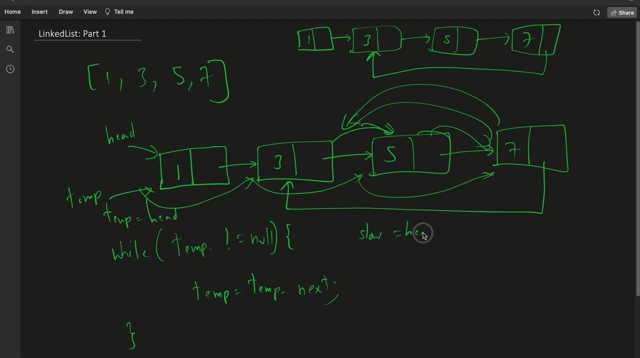 one as the slow pointer. we'll initialize it to help. we'll call another one as the fast pointer. we'll initialize it to help. okay, or temp already have has the value. so slow pointer points to temp, fast pointer points to temp. so right now this is slow pointing here, fast also pointing here when we move in a while loop. 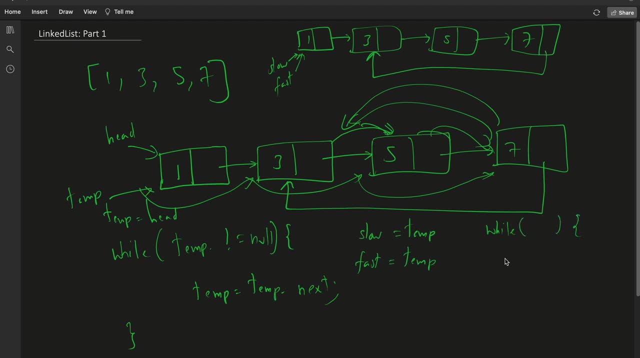 we will start by pointing the slow pointer. we will call another one as the fast pointer. we say: slow is equal to slow, dot next, it jumps by one value. and fast is equal to fast, dot next, dot. next, it jumps by two values. and if slow is equal equal to fast, so if ever they are both. 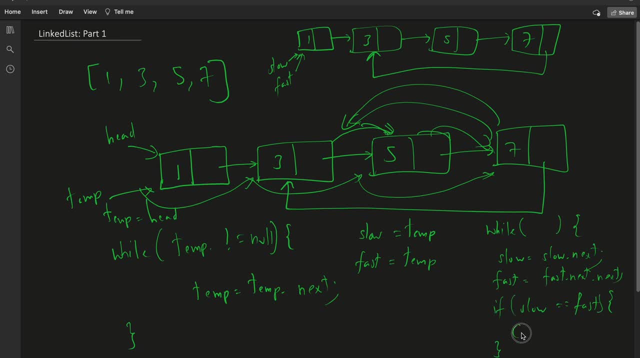 pointing at the same node. we can say: cycle exists, so cycle exists in this linked list. so let's see, for the example: slow pointer moves. let's keep their values here. slow and fast, right now both are pointing at one. now slow moves slowly. so by one value, slow dot. next slow comes here. so 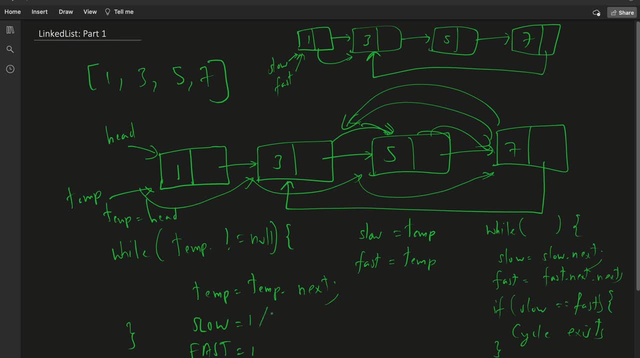 slowども statement is important because other interval isство pneuma starts from two points. slow is now pointing to 3, fast moves 2 values. so it's 3, 5, 5 is now at 5, slow then moves. 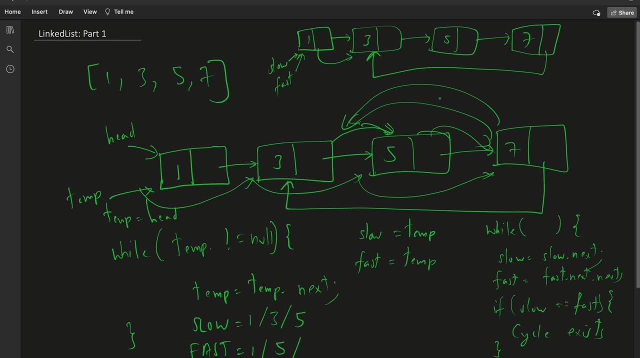 from 3 to 5,. 5 moves by 2 values, so from 5 to 7,, 7 to 3, so it came at 3, then slow moves to 7, and then fast moves from 3 to 5 and 7, 7,. at this stage slow and fast are. 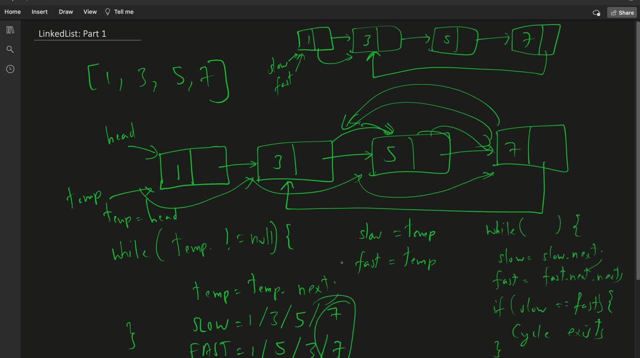 equal. a cycle exists, and this would happen in all the examples. so even if you consider another example, just for sake, let's see we have 1, let's delete a little. we have 1,, 1,, 1,. 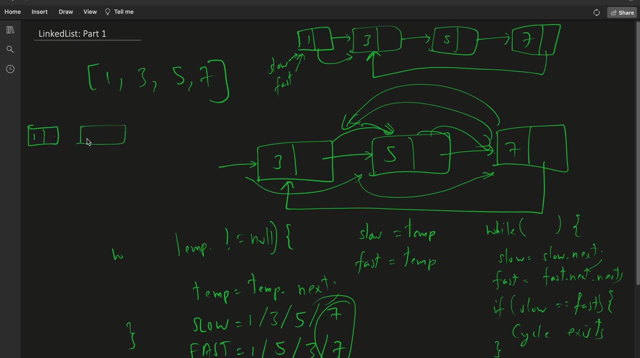 1,, 2,, 3,, 5,, 7,, 8. ok, I have added one extra value just to showcase that this approach will always work. ok, Now again we will do slow, fast, fast, fast. 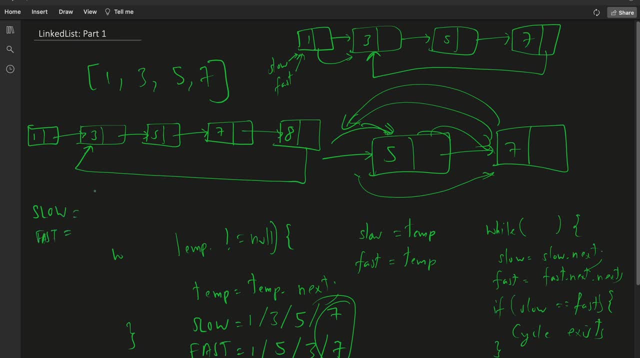 fast, fast, fast. So slow is at 1,, fast is at 1.. Slow moves by one value: slownext, it reaches the value 3.. Fast reaches the value 5.. Slow then reaches the value 5, from 3 to 5.. 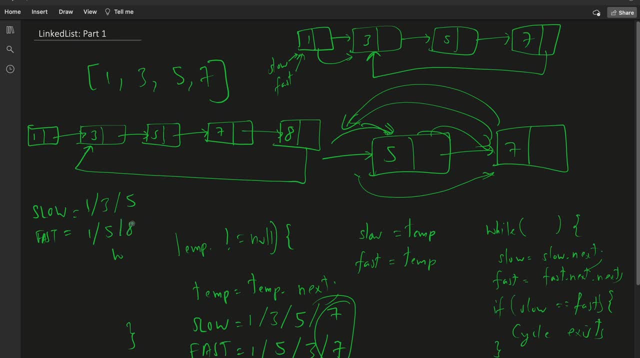 Fast reaches from 5 to 7, 8, so it gets 8.. Slow goes from 5 to 7.. Fast goes from 8 to 3 and then 5.. Slow goes from 7 to 8.. Fast goes from 5 to 7 and then 8, two jumps. 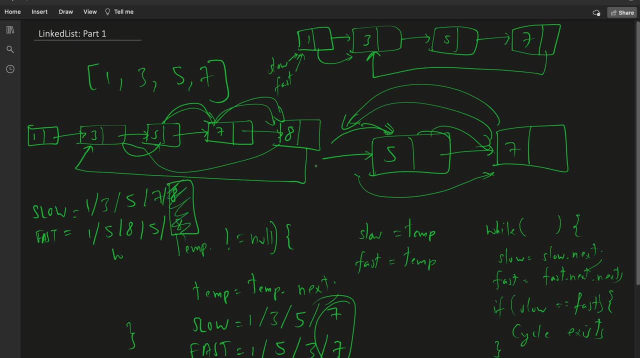 So at this point both 8 and 8, they match, So we can say a cycle exists. This is one of the most common examples. We'll cover them in the part 2 as well, But hope these things clear out your concepts on linked list. 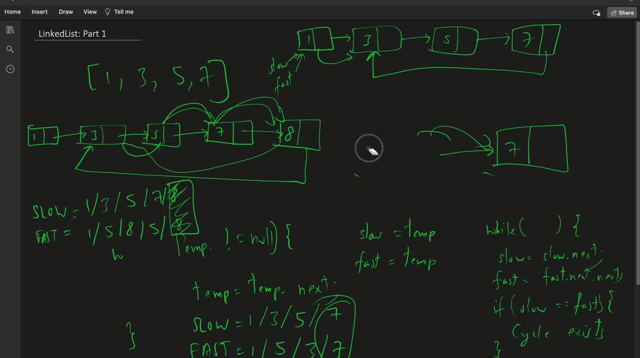 Now, before moving forward, there is one very important thing For you all to understand. If you notice carefully whenever we discuss that, arrays are stored in memory in contagious memory location, right? So if there is an array of size 4, it'll get continuous 4 memory locations, right? 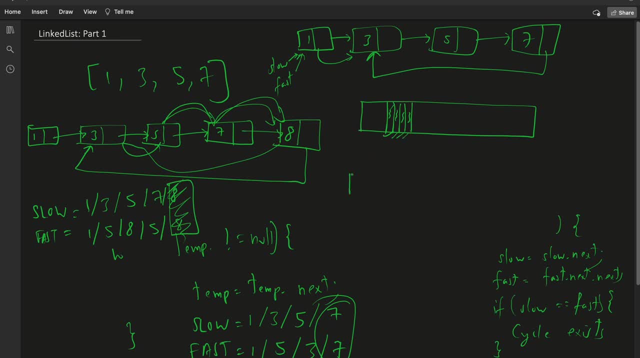 1,, 2,, 3,, 4.. And when we have a single linked list, what are we doing? We are storing data on one side and pointer to the next node. You can actually say that this is an array of size 2, because now, all the time, data and 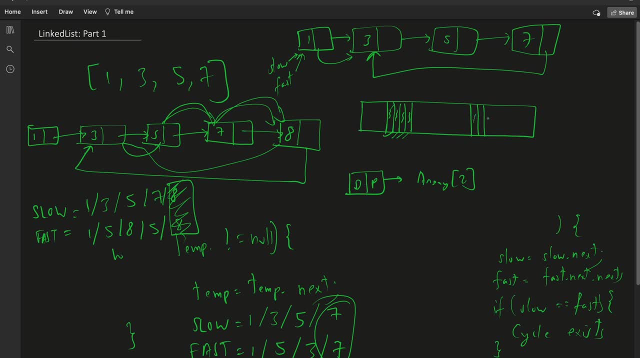 pointer to the next. they are in contagious memory locations And here, in this one, we store the value of the data, That is one, let's say, picking up from this, and in the next one we store the address of the another node somewhere, right. 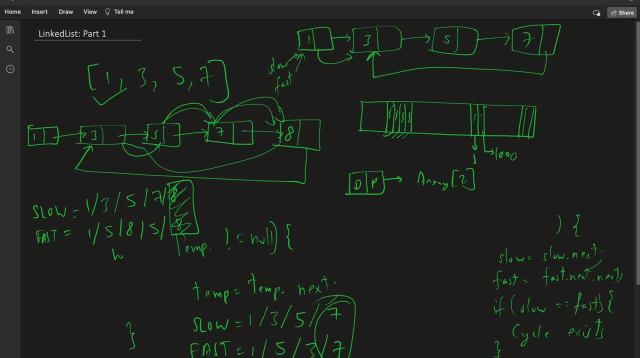 But that is also integer value. So even if I'm storing 1000.. 1000 as an address to the next node, I'm actually storing an integer value. So you can say linked list. you consider a single linked list is actually an array of. 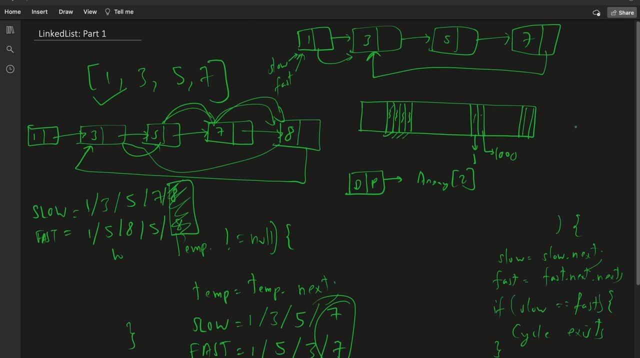 size 2, right, And you just create more and more arrays and you add the values. Similarly, w linked list is an array of size 3.. What if? now, this is why linked lists are called the fundamental data structures, And if you see, arrays are the fundamental data structures as well? 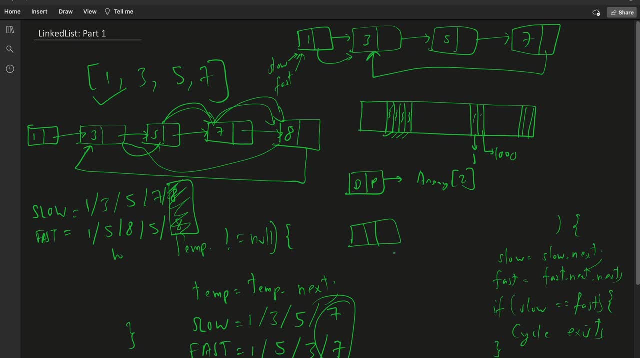 Because Arrays are being used to implement linked lists. Let's say you have a very customized problem statement, okay, where you have to store phone numbers of people. You can actually create an array of 11, 1,, 2,, 3,, 4,, 5,, 6,, 7,, 8,, 9,, 10,, 11,, 11 values. 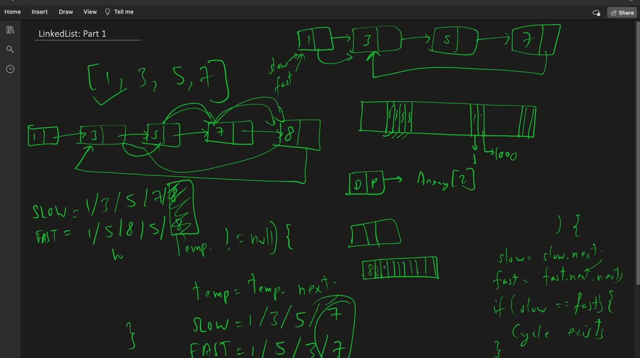 Okay, And those values would be phone number, let's say 8,, 2,, 5,, 4,, 3,, something like that. And the last one, We'll store the number of people. Okay, We'll store address to the next node that will again have 11 elements. 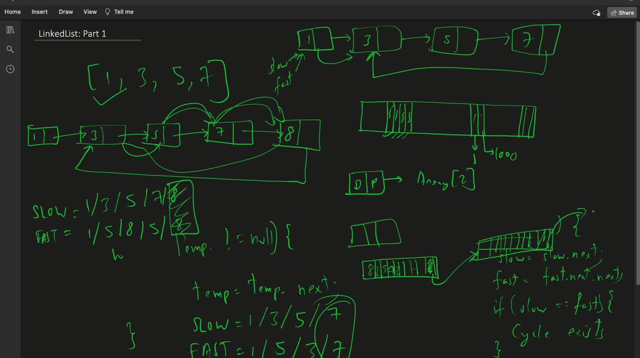 The first 10 are the phone number value and the next one is the node to the next one. But since Java does not allow us direct access to the pointer and their addresses- this can be done with C, So in Java we directly create them as classes. 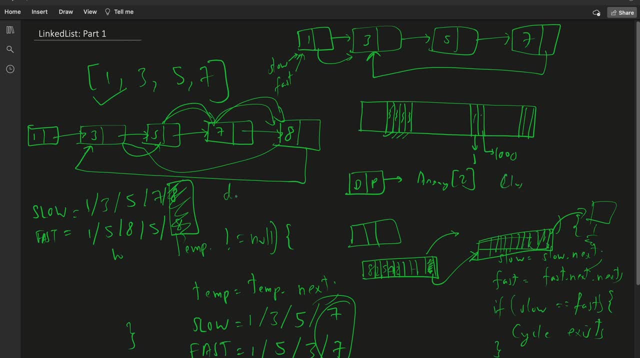 But again, as we create a w linked list classes where we store data, uh, then next pointer and previous pointer, you can actually store data, data two, data three, data four, data five, any kind of data structure, and then next, previous and anything. 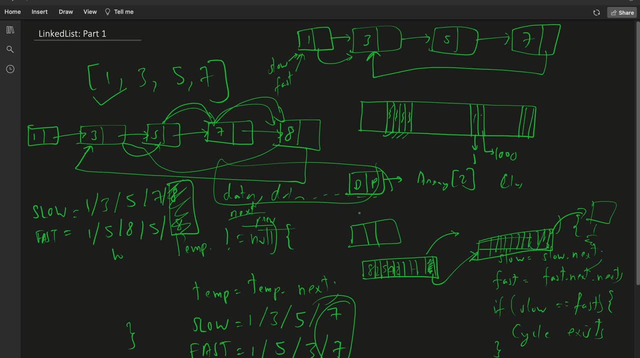 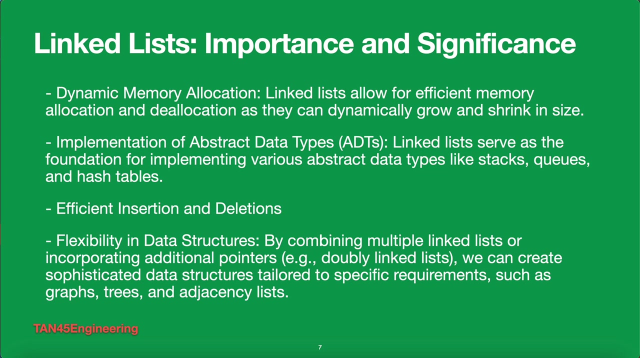 So, if you see, all data structures emerges from linked list and linked list emerges from arrays again. Okay, I hope this helps. uh, let's move forward. So um, in the end, uh, few of the importance and significance of linked list. 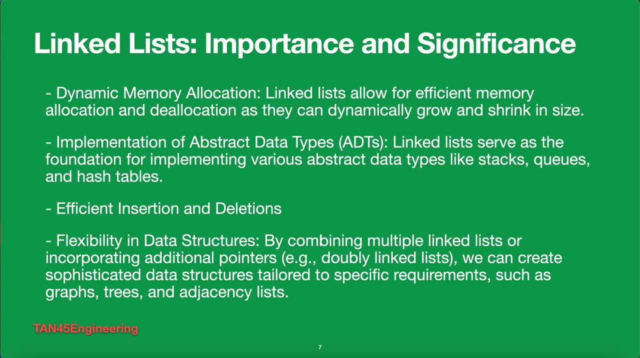 So dynamic memory allocation. Since you know that uh insertion and deletion is very possible, very easy with linked list, The dynamic memory allocation is really good. like in case of arrays, we need to know the size beforehand, but for linked list we can add elements after elements: uh implementation. 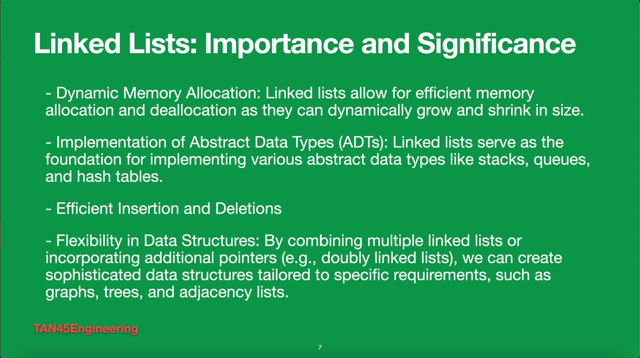 of abstract data types. So, if you see linked list, serve as the foundation, as we just discussed, for implementing various uh other data types like stacks, queues, hash table. In fact, if you go for uh binary trees, trees- 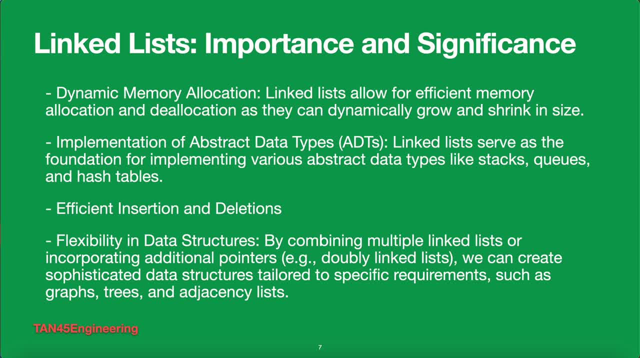 They, they all come from linked list. uh, very efficient insertion, ends and deletions, as we just saw. plus flexibility in data structures. by combining multiple linked list or incorporating additional pointers doubly linked list, We can create sophisticated data structures tailored to specific requirements, such as. 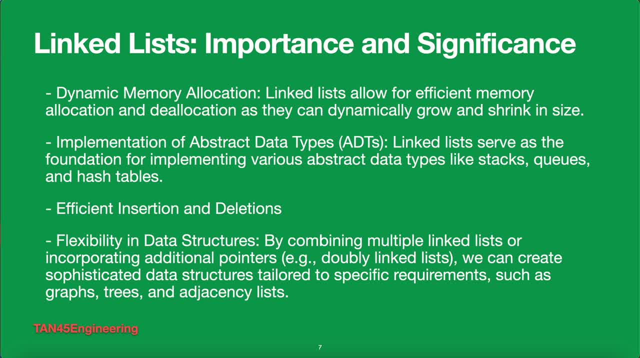 graph, trees, adjacency list and the phone number example that we just saw right. So linked lists are really, really important data structure when you're starting your journey on data structures. So if you have an algorithm, linked list and uh arrays, implementations, their theory. 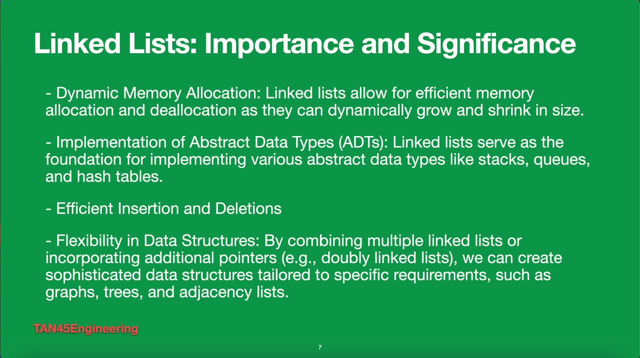 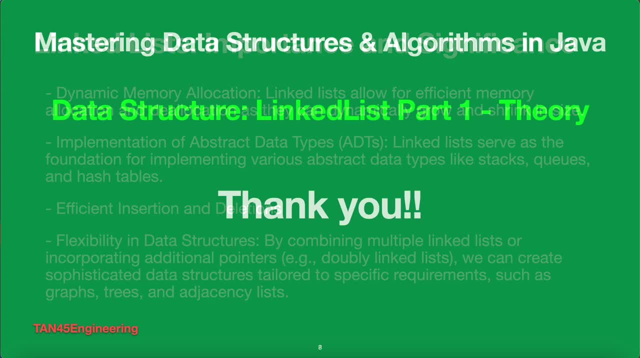 the fundamentals and their understandings become very critical to this journey. Okay, So please go through the video again and understand them well enough In the end. Um, that's all from today's video, everyone. uh, for the next video. uh, we'll cover the.